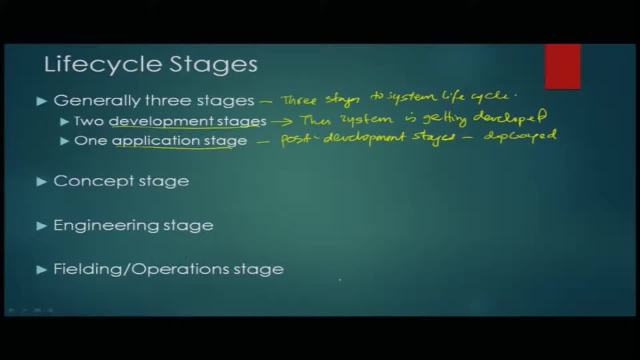 stage or the deployment stage of the system. So most of the models will have these three general stages and the stage. the first stage is usually called as a concept stage and the concept stage we can define it as the. it is the initial stage, initial stage of any given. 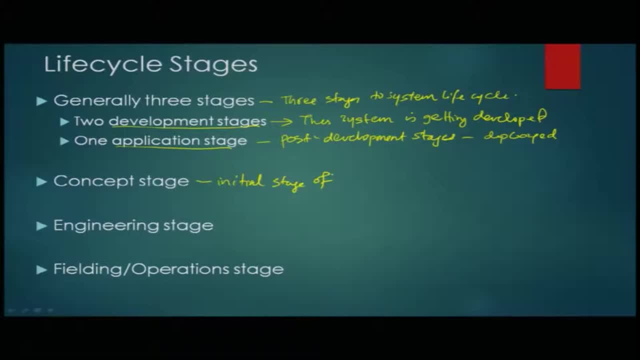 model. Okay, So system formulation and system definition: formulation, system definition and system definition that will best satisfy the customer need. The importance here is that we are talking about the formulation of the system and the definition of the system or system concept definition, or you can think about it as system. 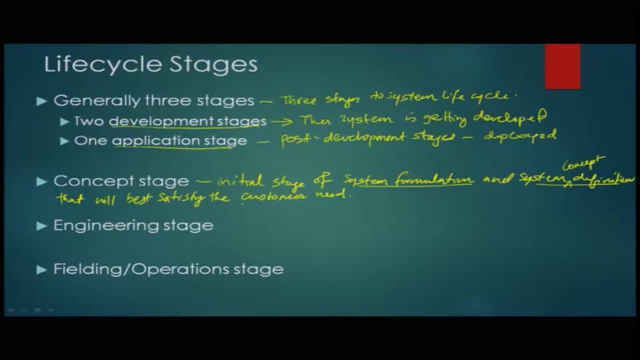 concept definition that will best satisfy the customer need. The important thing about the customer need is that this should be available. There should be some validity behind the need and many then certain models. this stage is also called as system architecturing. So when somebody is talking about system architecturing, it is the initial stage of 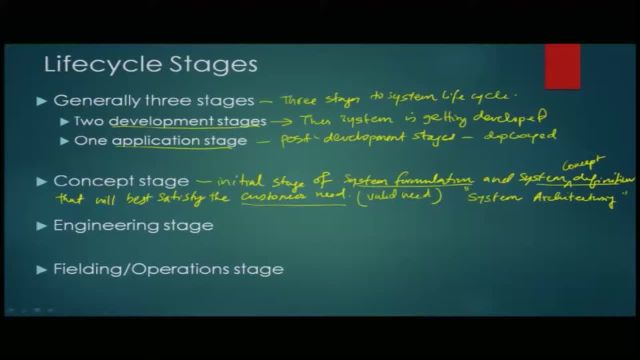 the formulation and the concept definition of the system where we are trying to satisfy the valid need of a customer. The engineering stage is the second stage, where the second stage- this is again a stage of development. So these two are the development stages. 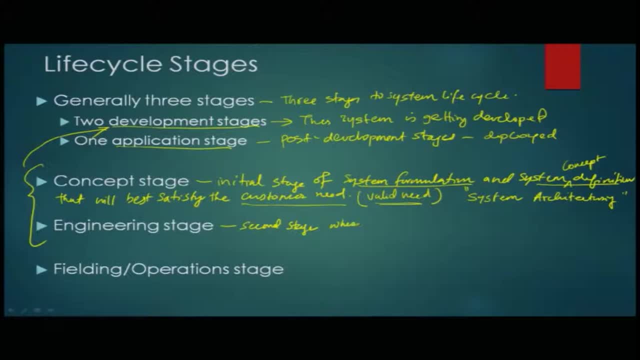 In the second stage, where the system concept is translated into a value: Hooker standard definition. physical system design- physical system design. again, we are talking about the physical system design here because our work is more. our discussion is mostly about the products that are to be. 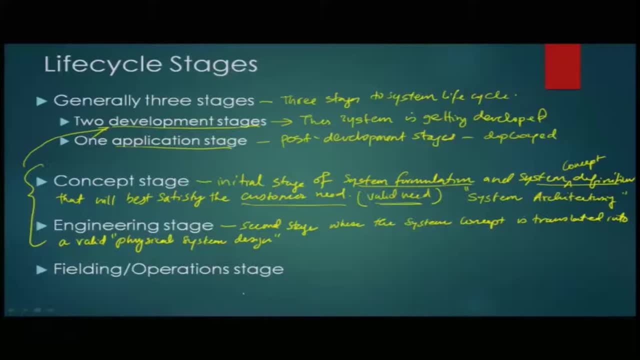 manufactured or systems that are manufactured. we are not talking too much about soft systems or software systems. so the physical system designs. what design is it? the that fulfill that fulfill the requirements of the customer within reasonable cost and schedule? reasonable cost and reasonable cost and reasonable cost and schedule. 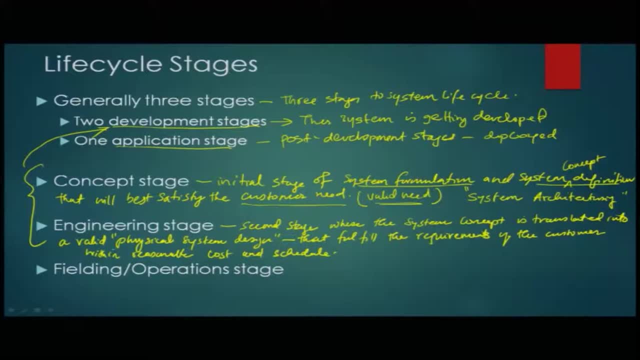 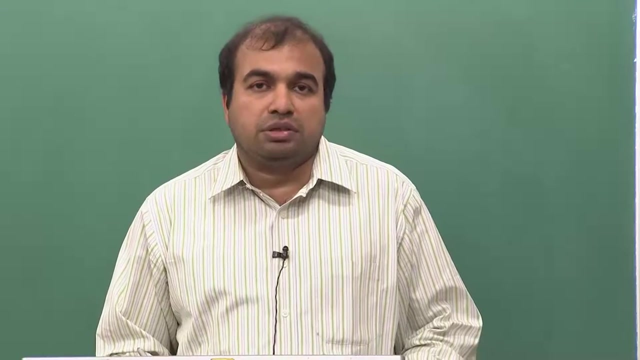 So here we are translating the concept into a physical system design. so physical product is being designed and built or engineered which will fulfill the customer requirements within reasonable cost and schedule. so nobody will be interested in designing a system which is with unreasonable cost and unreasonable schedule. 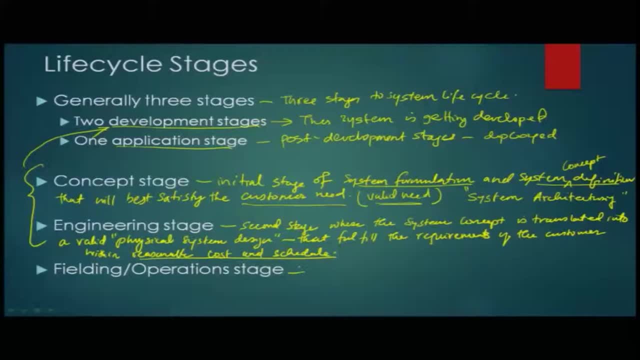 So that is the important aspect of this. and then the third phase of the system, which is the fielding or the operation stage, or what we call as the application stage, or sometimes also known as known as post developmental stage, as I said earlier, because it is after. 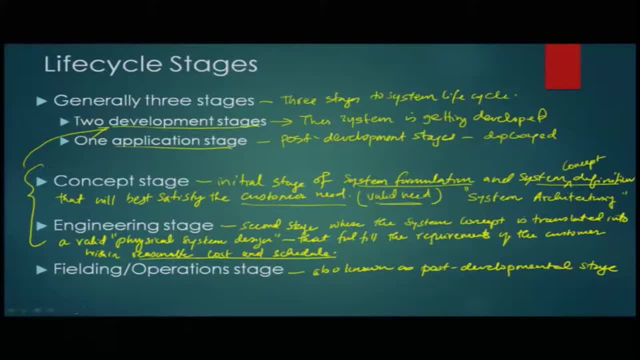 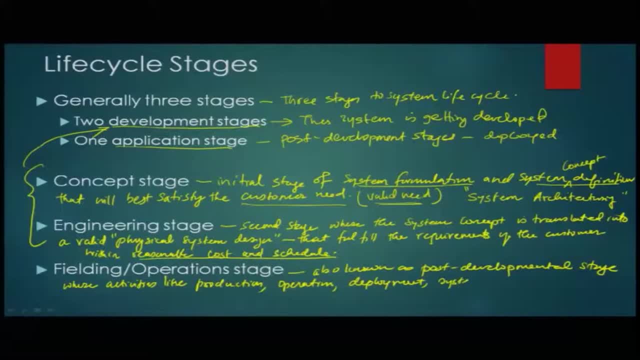 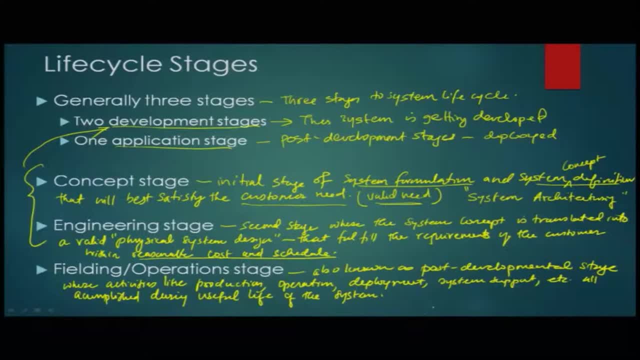 Production. thirty minutes to go. So here the system is in the what we call as the fielded stage. it is doing what it is supposed to do. what is supposed to do? So the assistance provided here is also one comes as under the application stage of the. 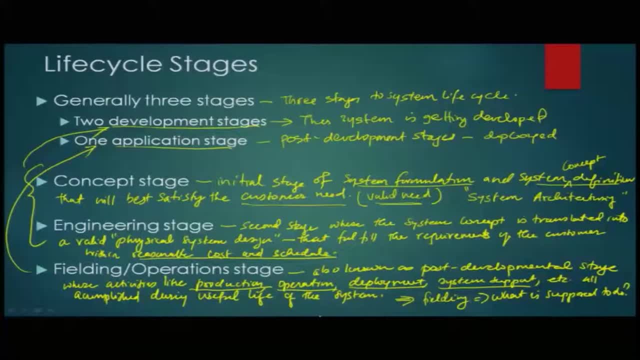 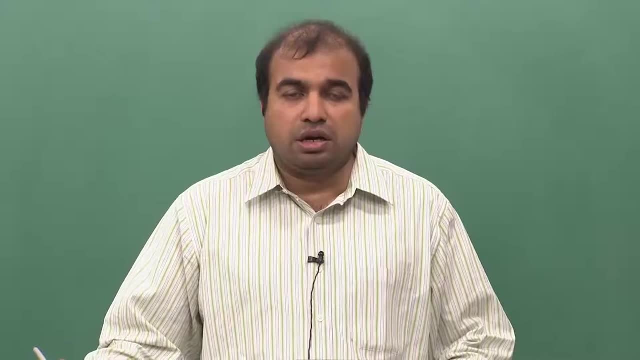 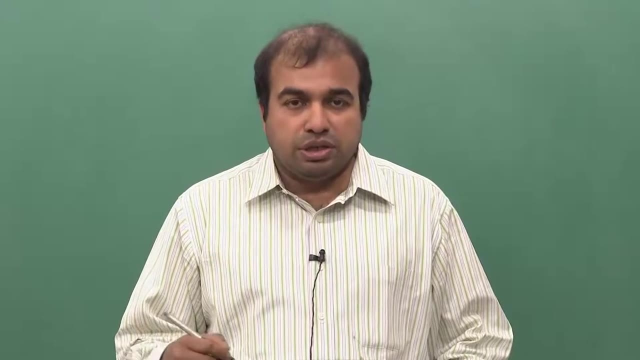 system. So these are the three major stages in almost all systems engineering- life cycle stage, life cycle models- and you will see different variations and permutation combinations of stuff here. So what we will do is that we will look into detail of these three stages and try to decipher. 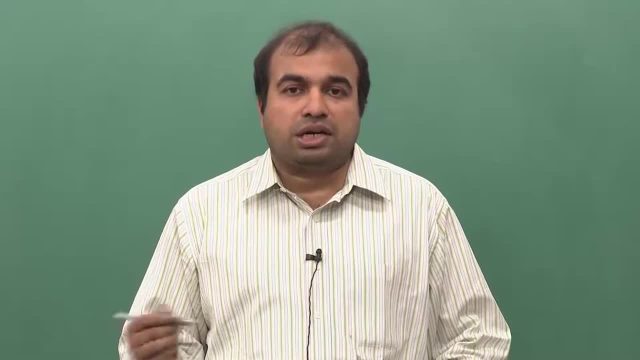 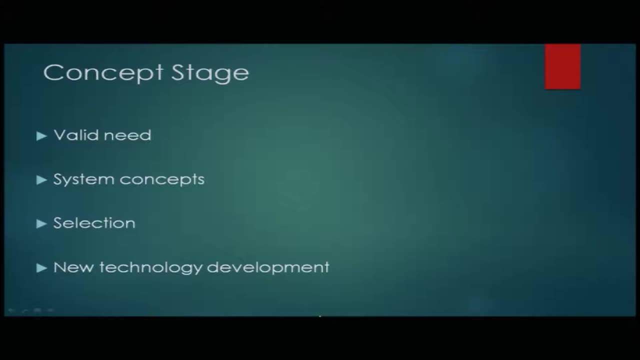 what are the things that constitute these stages and what are the major activities that are part of these stages? So, the concept stage, the first thing that we need to talk about is the concept stage, and if you think about a concept stage, it, this stage, comprises of: 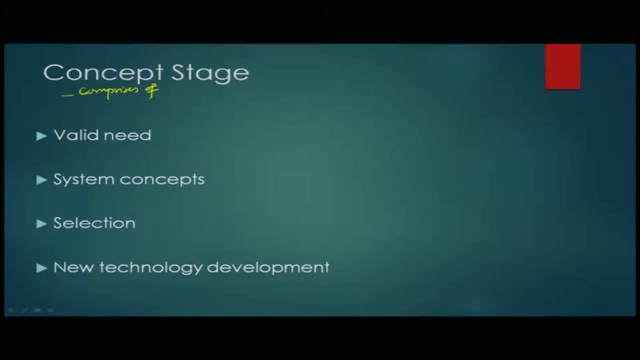 An architecture of who, an architecture of the system, and that is realizable. so what are we talking about? this point? we are also trying to establish the possibility or feasibility of an architecture. is it actually possible to design the system and that architecture? is it realizable? 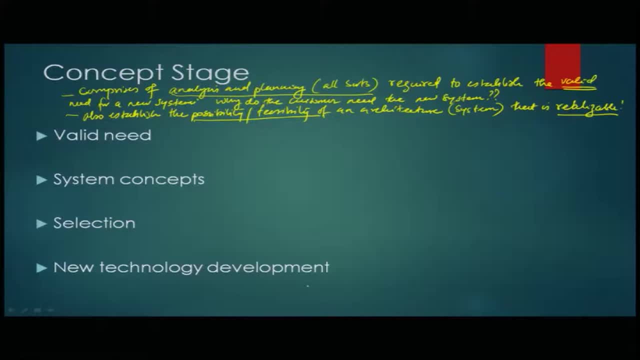 So those are the two aspects, okay, and in the way that all of these things together satisfy the need in the best possible way, okay. So the concept stage is it comprises of all analysis and planning, All type of analysis and planning required to establish the valid need of the new system. 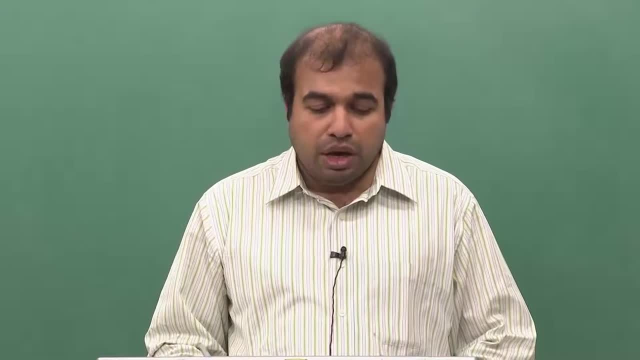 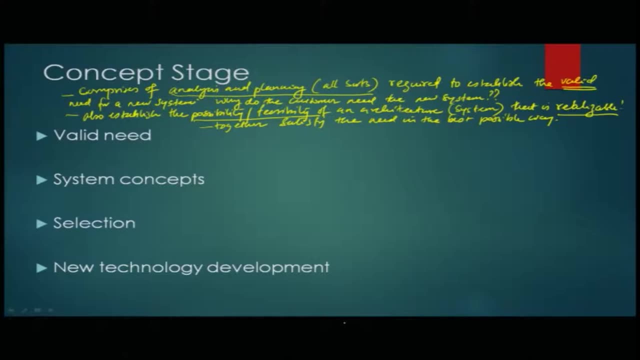 or you are answering the question: why do the customer need the new system? Also, along with that establishing the need, you are also establishing the possibility or feasibility of an architecture of this or possibility of a system, architecture that is realizable or that can be realized within a reasonable cost and a schedule, with the 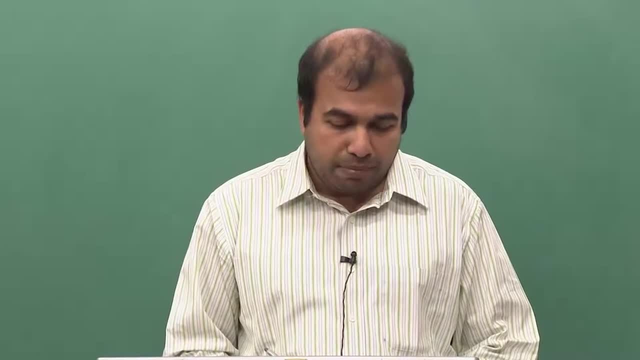 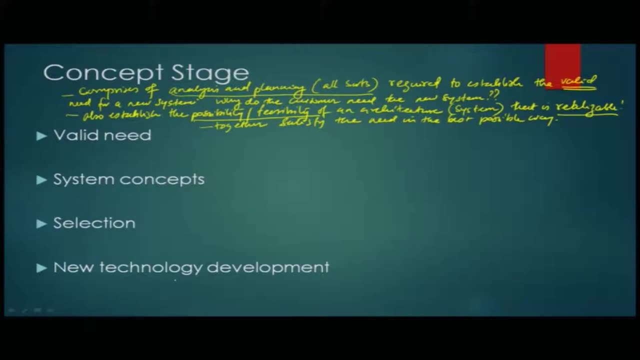 so that the customer need can be satisfied in the best possible way. So the first characteristic, as we talked about it, is the valid need. So what is a valid need? So the valid need is? so we here is that we are establishing that there is a valid need. 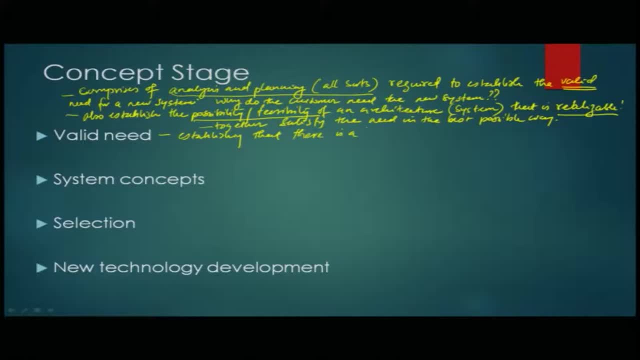 there is a valid need, or you can also think about it as a market feasibility- So if you make the product, there will be somebody to buy this- And for the new system. so there is a valid need for the new system that is technically and economically feasible. 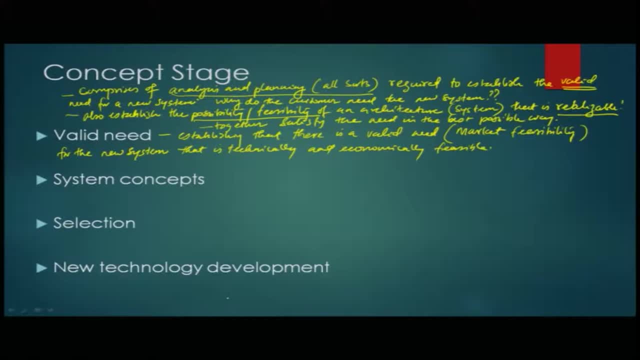 So what we are saying here is that you establish the valid need and also establish the technical and economical feasibility of the need. That is the first aspect of the concept stage. you are establishing the validity of the need. Then we talk about the system concepts, which is the second aspect. 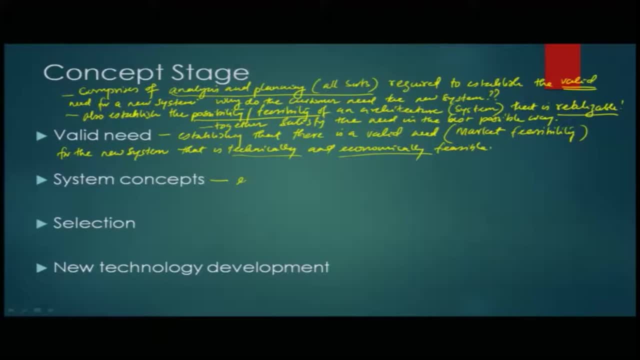 So the system concepts here is that you are exploring. the establishing was the first part. here you are exploring potential system concepts, potential system concepts Or formulations, system concepts or formulations along with valid sets of system performance requirements. So here you are exploring multiple concepts, Multiple potential system concepts or formulations. concepts or formulations are they are like. 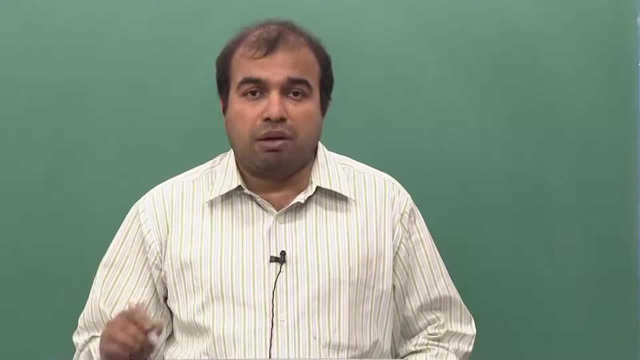 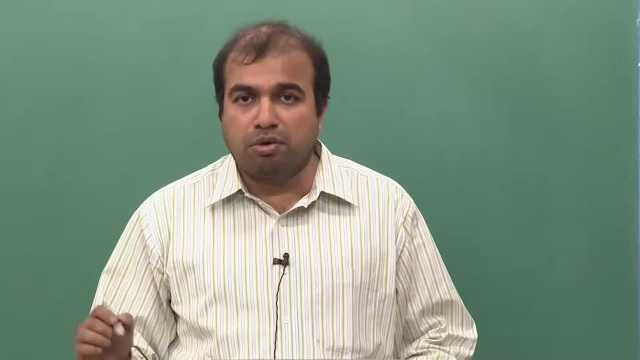 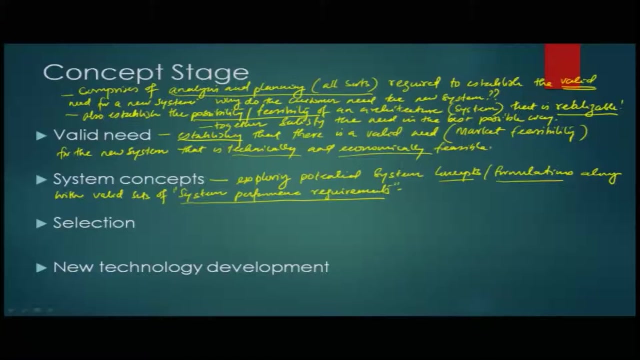 us. we send in one of the presentations. all of these are black boxes. we are not really detailing the circuit diagrams or the interfaces or anything like that, But these are basically the major blocks- building blocks of the system and, along with the valid system, performances. So what we are saying here is that the system should be able to meet these performance requirements. 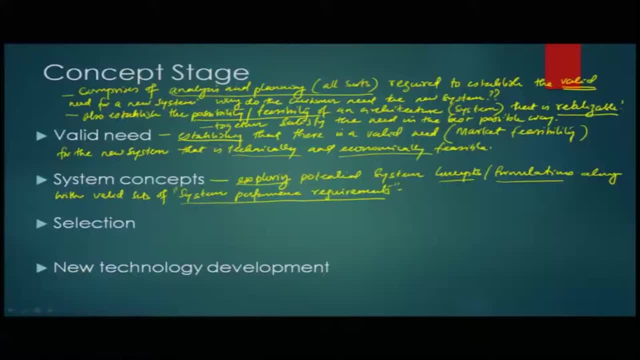 that is the system concept. So the exploration is the Second aspect of the concept stage. Then third aspect of the concept stage is the selection. So here is the selection, selection of the most attractive system concept, The attractive term. it is not about the beauty or attractiveness or something it is about. 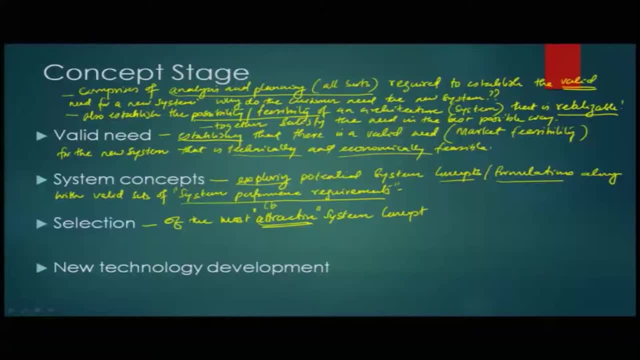 the best fit, So the attractive. we can think about it as a best system Suited Kind of a concept, So the best suited system concept, And then Define the functional characteristics. Define the functional characteristics, Characteristics for physics of what, of the attractive system concept. 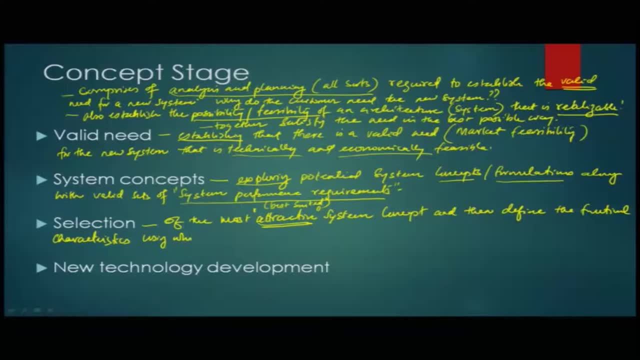 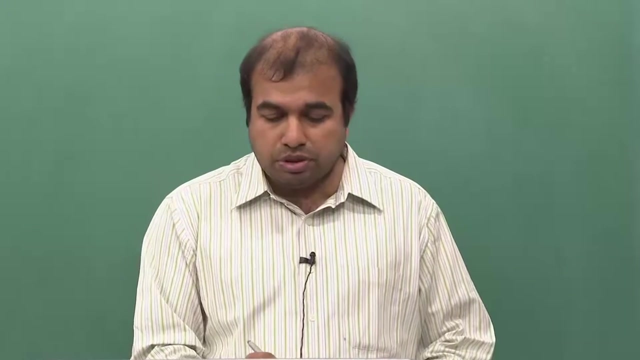 Okay, Using which Engineering, Production And Operations Plans Can be made. So here The best suited system concept. So here is a selection process. from the explore the potential system concepts, you choose the best suited or the attractive system concept. 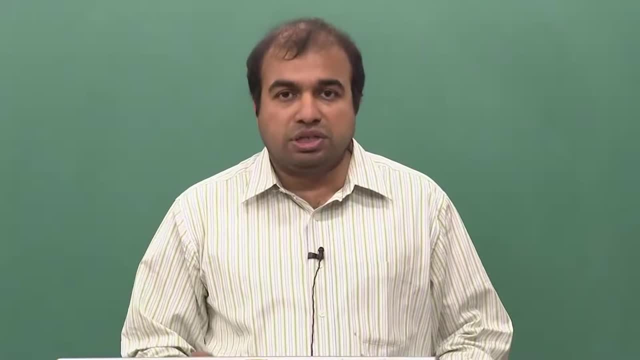 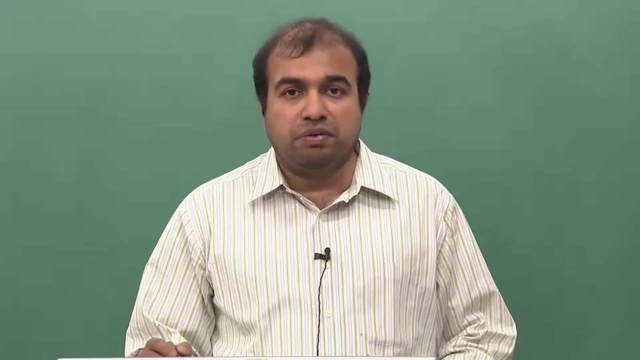 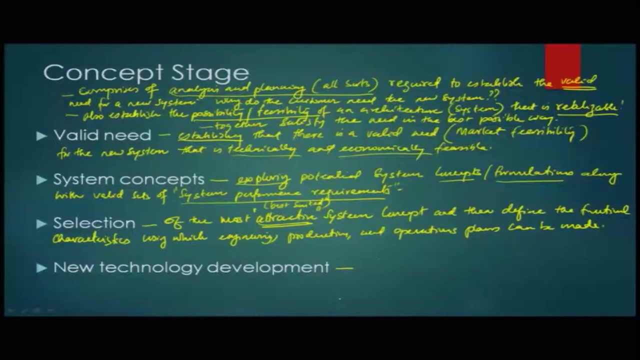 And Define the functional characteristics of the concept in such a way that the engineering, production and operations plans can be made using the concept definition, the selected concept definition that is just created out of this. Then there is another aspect, also called as a new technology development, because 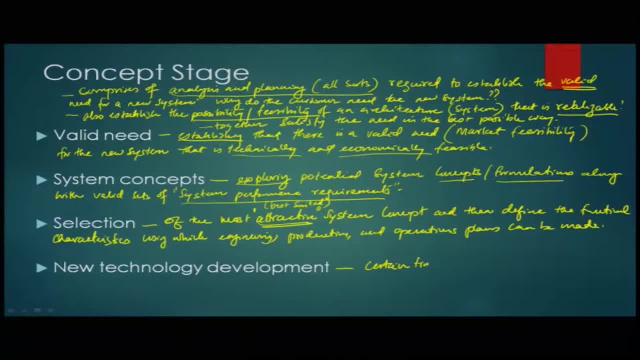 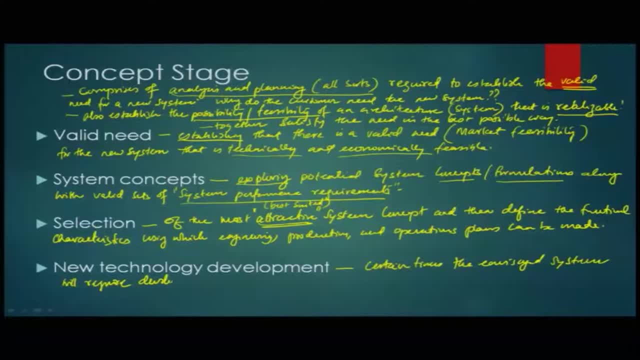 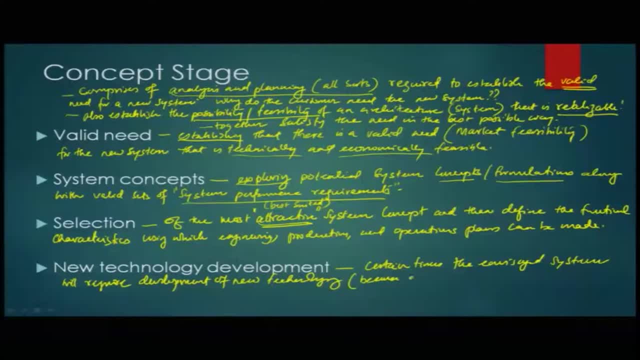 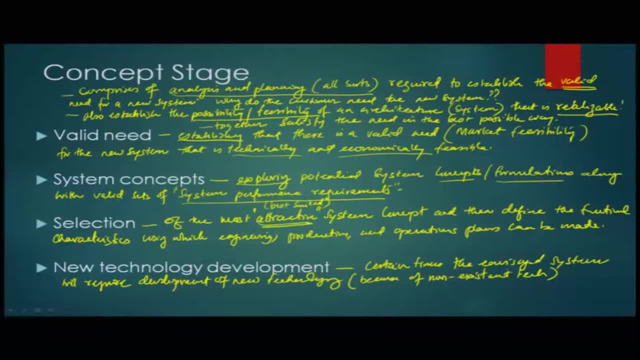 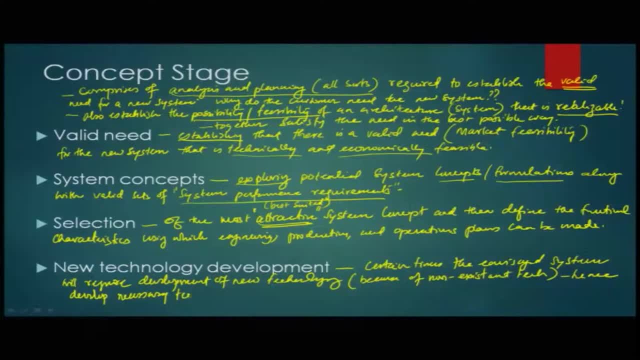 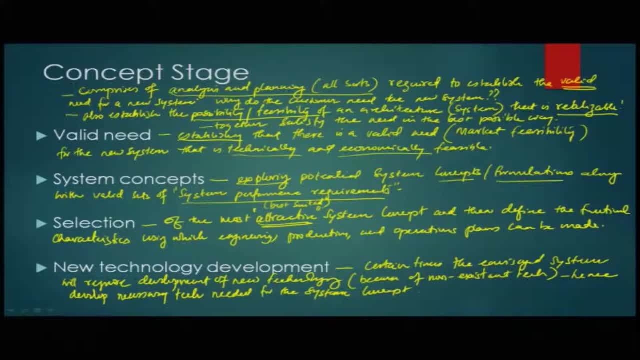 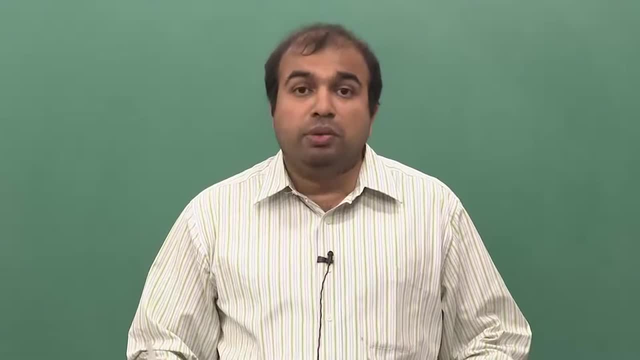 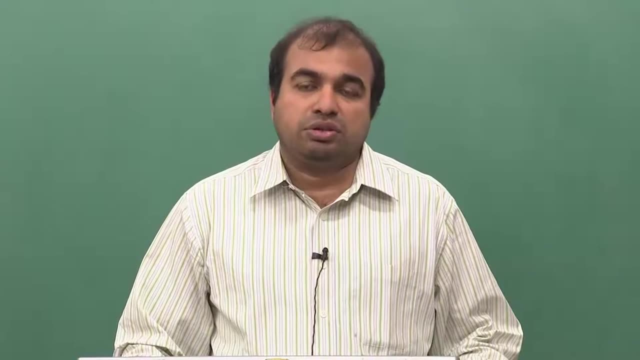 Envisaged system. Envisaged system. Envisaged system. So if a new material is necessary- for example, when Rolls Royce designed the trend series of engine, trend 1000 series of engine, they were looking for new materials for the fan. 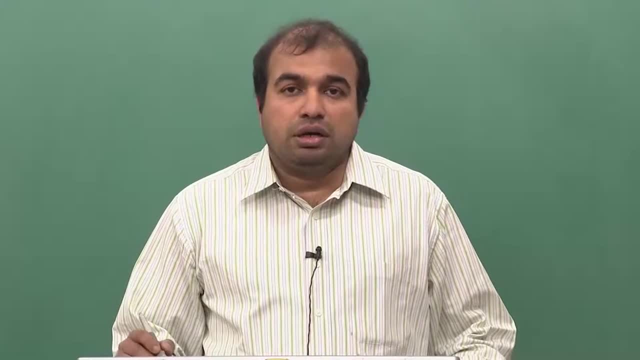 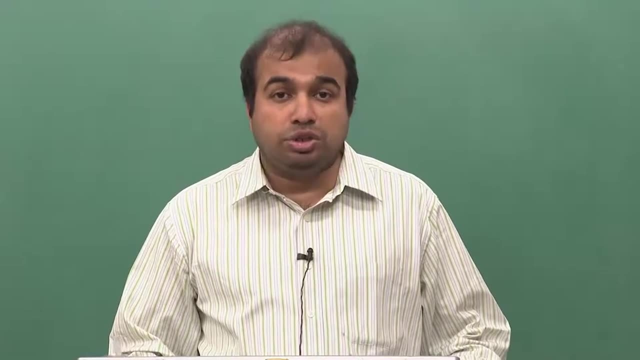 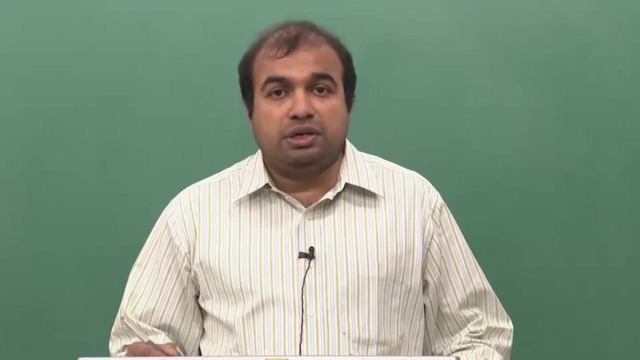 blades and that actually required, and they finally choose the material as titanium alloys, and it required a new manufacturing or fabrication technology to be developed as part of that process, and hence that was developed by Rolls Royce. So, and then they developed it, tested it and proved that the fan blades that are built 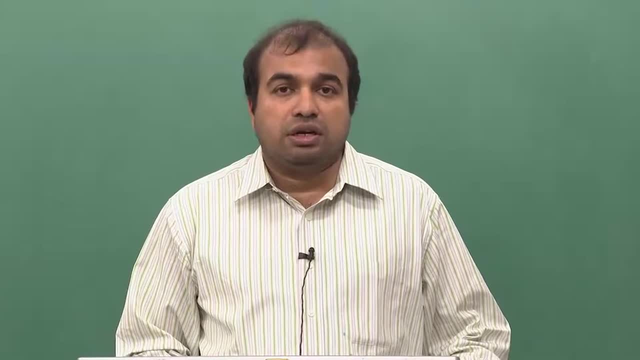 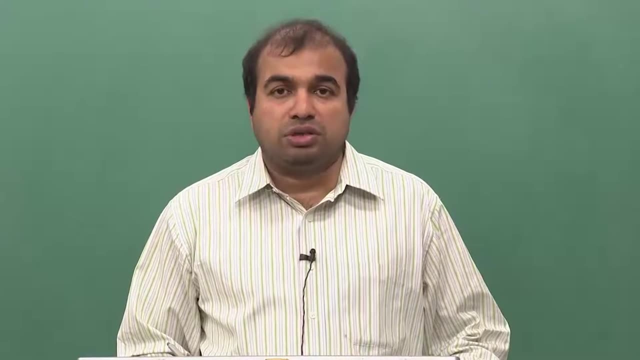 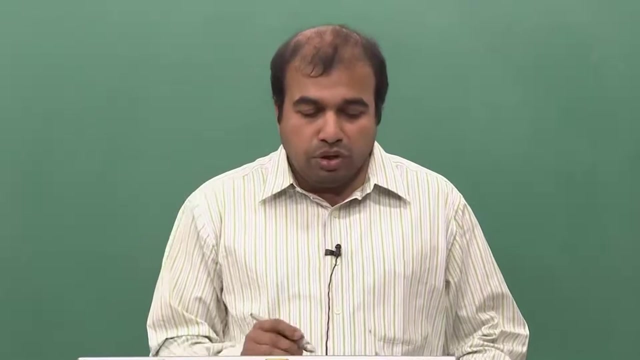 using the technology. new developed technology is in fact actually better than the existing process. So these kind of new technology sometimes will be required as part of the system concept and if it is necessary, then that new technology development also becomes part of the concept stage. So when you go through all these four aspects of the concept stage- as in certain cases you 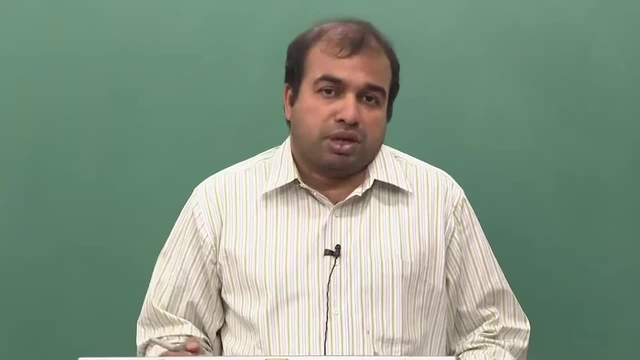 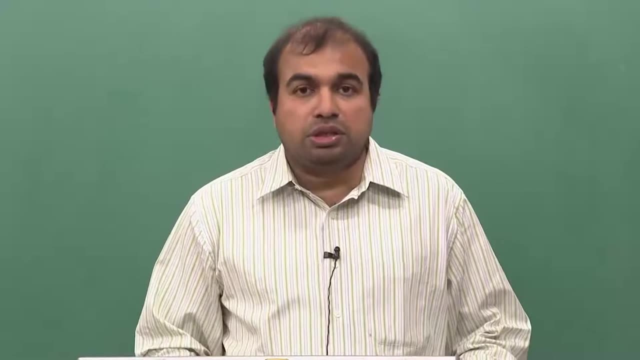 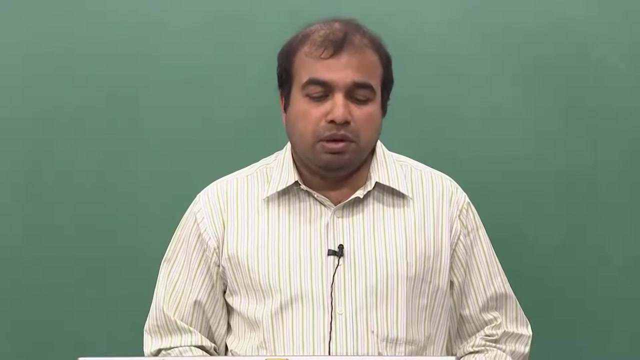 might only go through two, certain three, certain times you might go through, because sometimes you might not require a new technology development. all the necessary technology is available. So then you will only end up doing the three aspects of it. but anyway, within these four aspects, with different permutations and combinations of these four aspects, you would be able to. 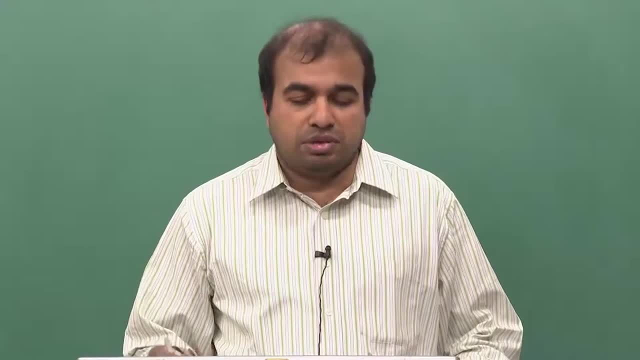 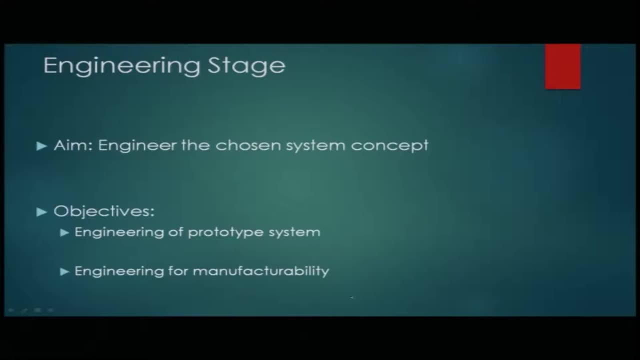 come up with the reasonably good concept of the system, which is the output of the system concept stage. Then comes the engineering stage, the second phase, after the engineer, after the system concept. So, as I said earlier, the aim of it is to engineer the chosen system concept. 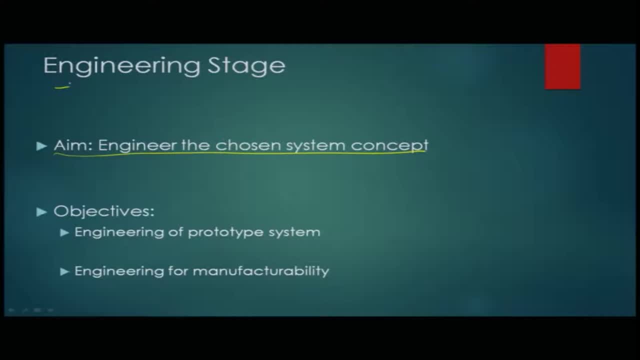 So the engineering is actually in. if you think about it, it is actually the development of a physical system, system from where do you develop? from or based on the chosen system concept, Chosen system concept from the previous stage and so that the new system can be produced. 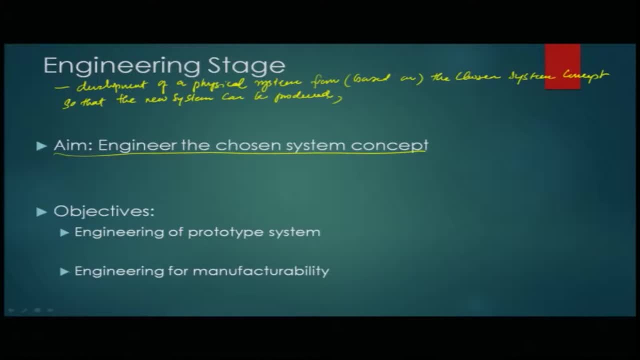 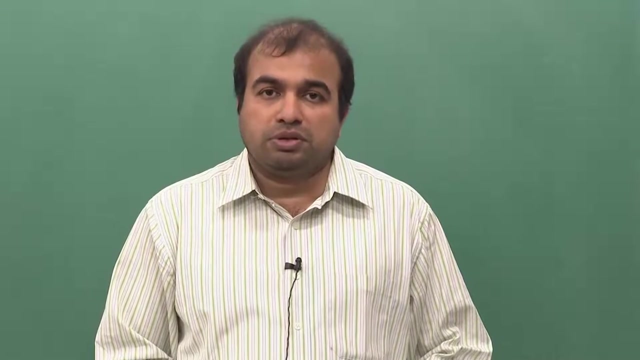 you can produce a new system. you can produce a new system, operate and maintain. How do you do produce, operate and maintain? all these things should be done economically and successfully. So the cost, economic aspects, economic viability and as well as the successful aspects of the system is also considered in this case. 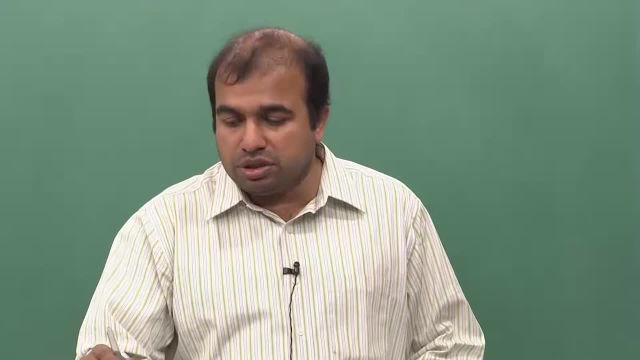 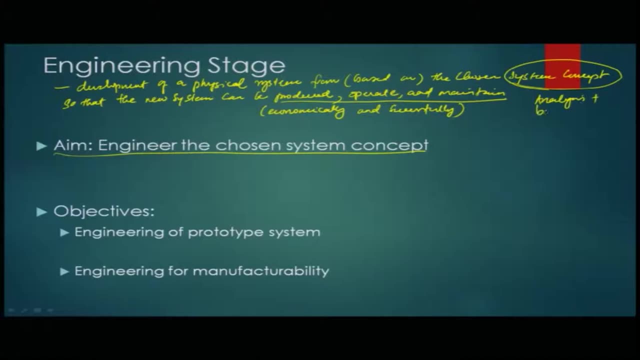 So you are the physical chosen system concept from the previous stage, which was more of an analysis plus basic aspects. From here, a physical design, a physical system is designed out of this one. So you are creating the physical product that can be produced, operated and maintained. that 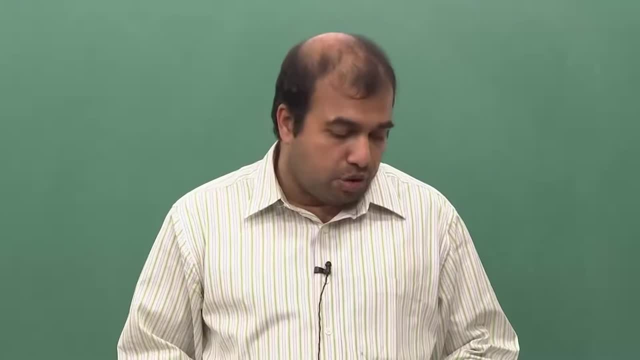 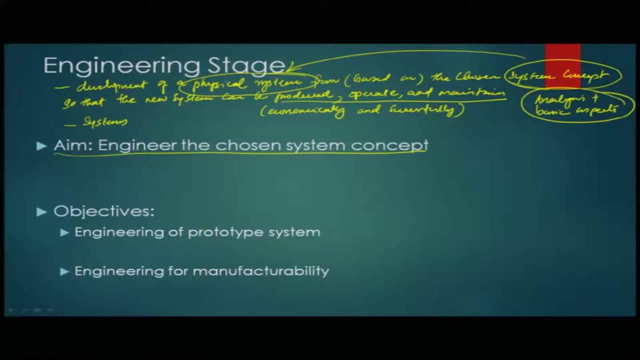 is the engineering stage of the life cycle model. Also, it should be noted that the aim of systems engineering, The life cycle model, should be noted, that the aim of systems engineering, systems engineering- We have mentioned this earlier- aims to guide the engineering process. 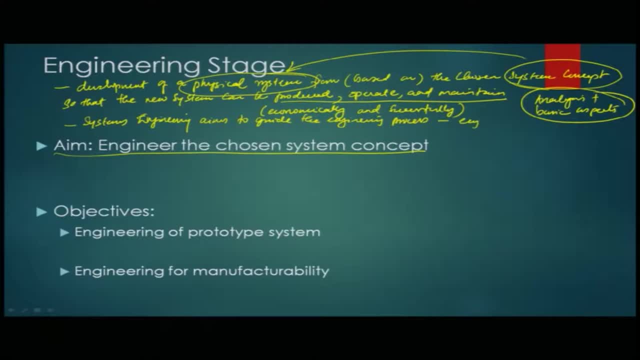 The engineering activities will be why? Because engineering will be done by experts. Engineering is not the job of the systems engineer. Systems engineering job is to guide the engineering process, because experts will do the engineering, and also to involve in design and management of interfaces, develop test cases and solve. 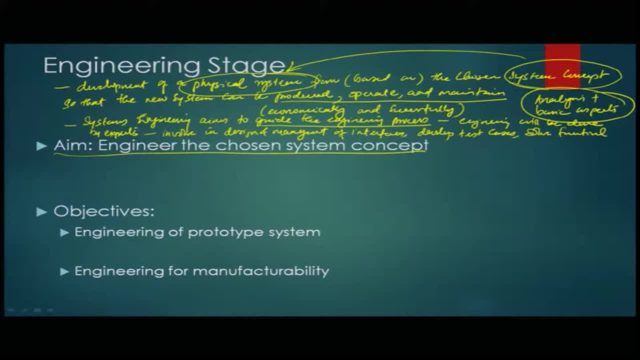 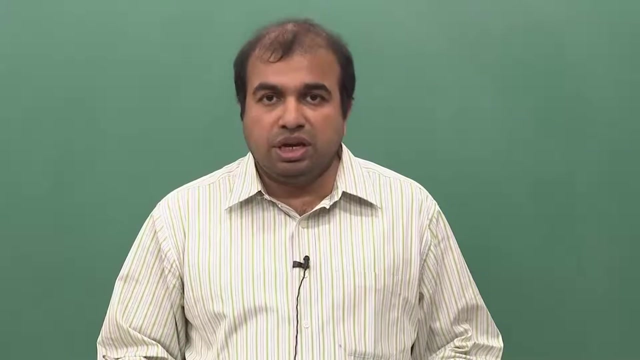 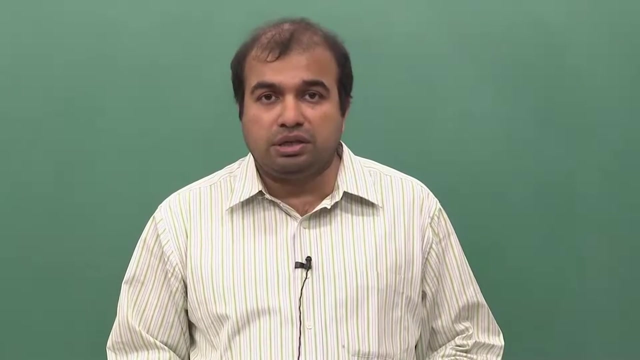 discrepancies, Solve functional discrepancies, Solve functional discrepancies, discrepancies, etcetera, are also aspect of the systems engineering. So the engineering stage, the role of the systems engineering, is to guide the engineering process, which are conducted by experts in appropriate disciplines, And also the systems engineer, in addition to guiding the engineering, will also be involved. 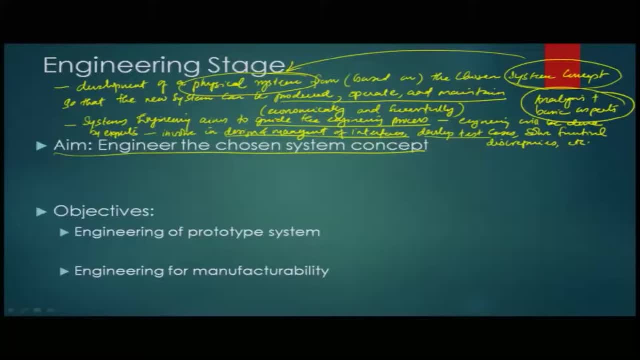 in the design and management of the interfaces. it will also be involved in the development of the test cases. Solve functional discrepancies. Solve functional discrepancies. So we look at it, the two main objectives that we talked about. it is okay. So the, as he said, the chosen system concept get translated to a physical system, okay. 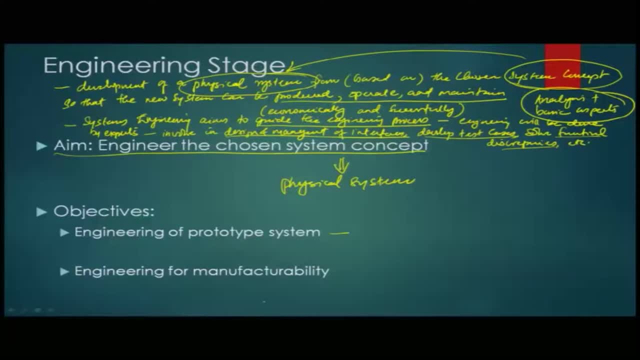 So the objectives is engineering of prototype system. So when we talk about a prototype system, the prototype that satisfies or implements- okay. So when we talk about a prototype system, the prototype that satisfies or implements okay. We can use the word fulfill also is fine. 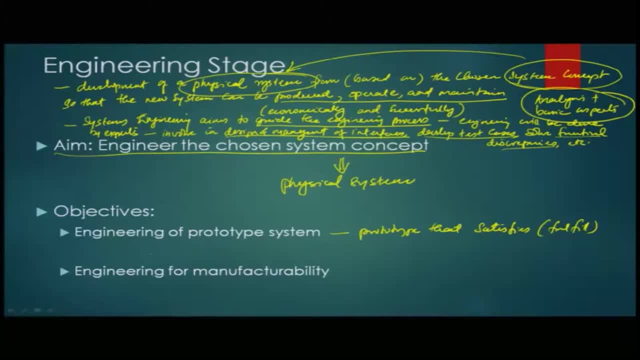 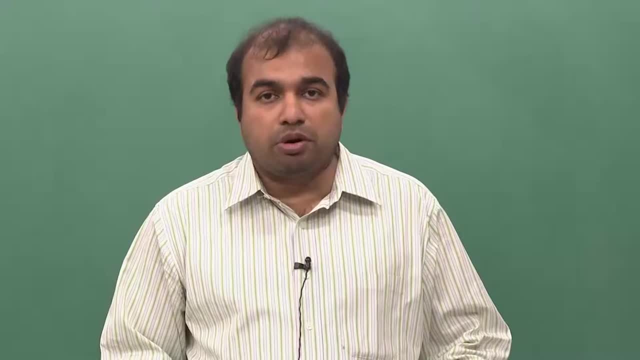 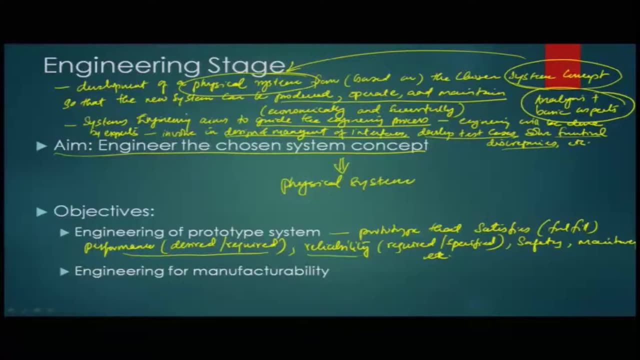 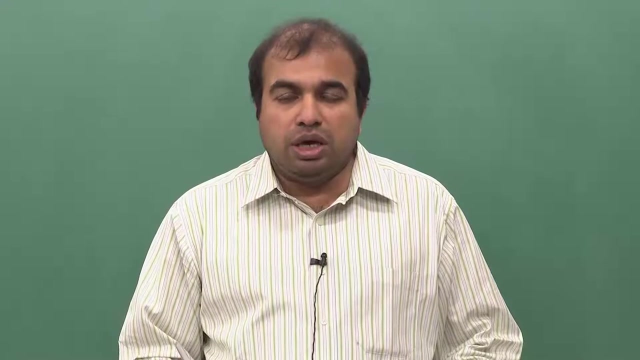 So in this case you are talking about not just designing any prototype, the prototype that satisfies or fulfill the performance requirements, the performance requirements, liability requirements, safety requirements, maintenance requirements, etcetera. So here, the physical system, the choice of components, interfaces, all those kind of things. 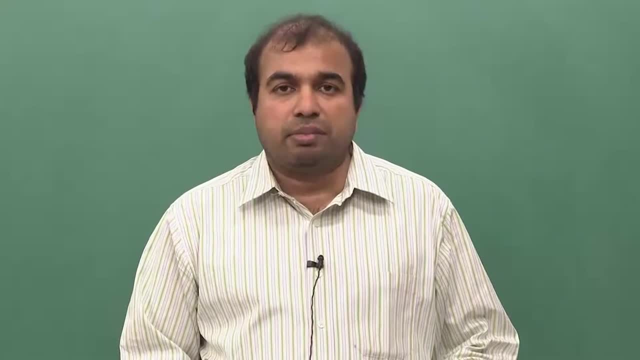 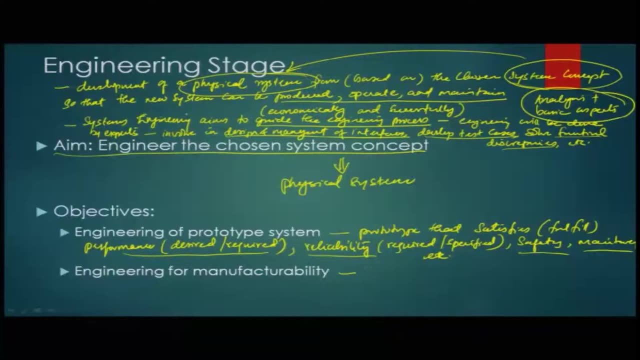 comes as part of this. the aim here is to satisfy the requirements and second aspect is engineering for manufacturability. So here is also- this is a concept, because some people different from the design for manufacturing- the aspect here is that ensure or ensuring economic production and usage. 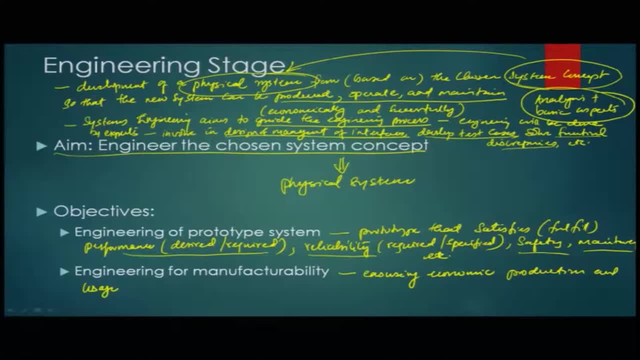 Okay. Or in a way ensuring affordability by the customer. So you don't want to create a scenario where you design a physical system which is not affordable by the customer. So the affordability, the economic production and usage is an important aspect of it. or in a way in the engineering stage. 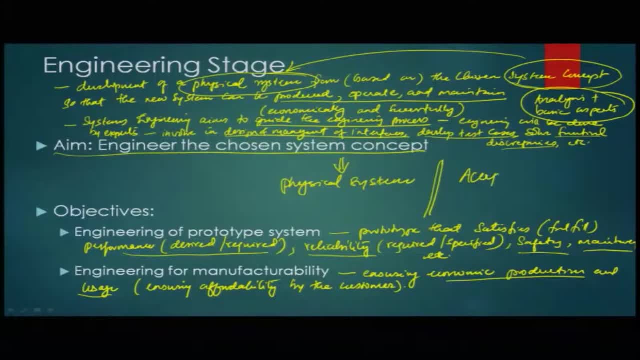 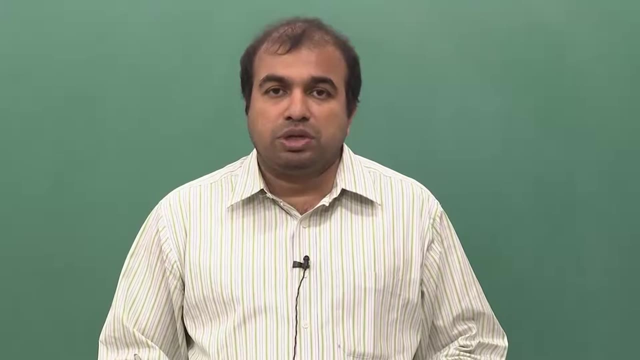 That is why. So you call this as the acceptance testing stage. So whatever the concept is, when you translate it into a physical product, then it should be acceptable to the customer. So that part, the acceptance to the customer, because the customer will only accept it if 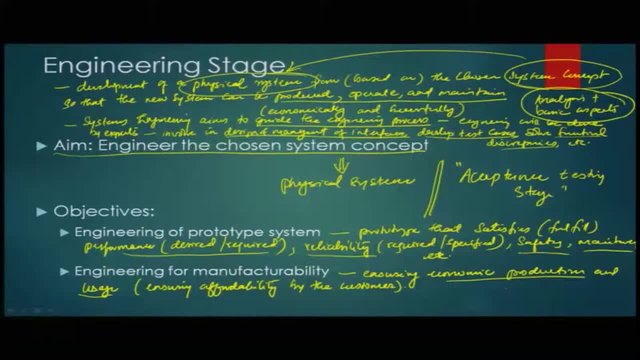 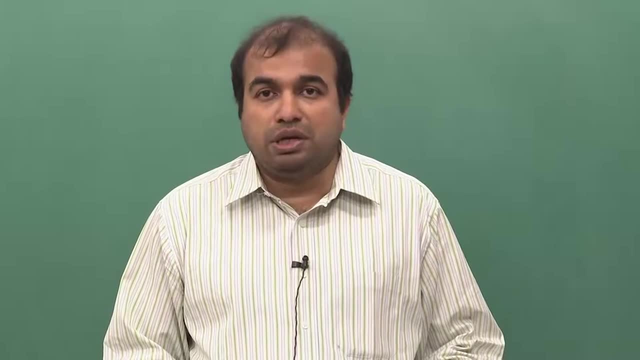 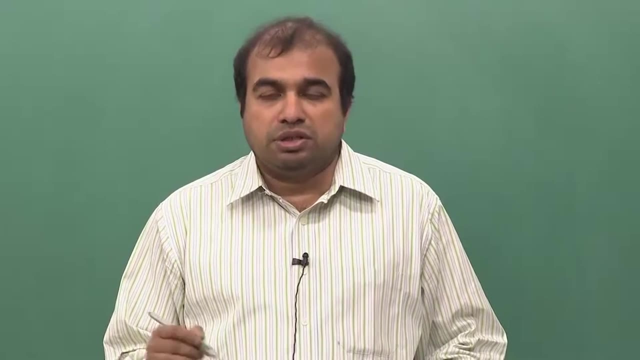 it is economically feasible to him to produce and use it. otherwise customer would say that is not an something that I am not. I am not interested in because I don't have the financial resources to maintain this. So that is the second aspect. So we now seen both of the pre-development phase. this is where actually by the end of 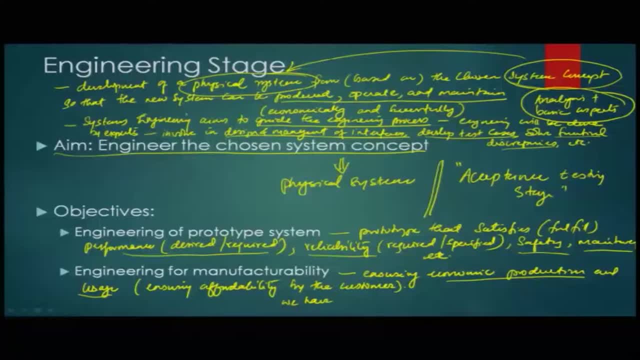 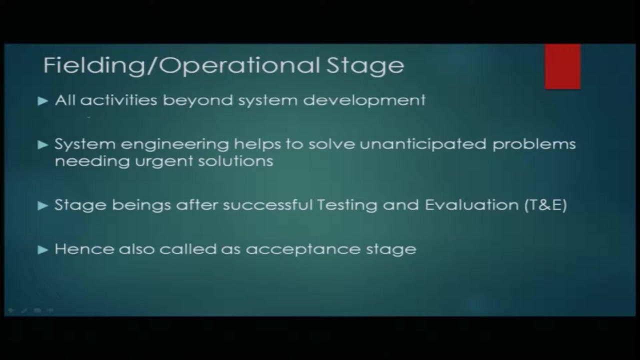 this stage, we have a physical system by end of this stage. that is the important aspect of this life cycle stage, Okay, Okay, Then the third part we talk about is the fielding and the operational stage. The fielding and the operational stage. this in a broad sense, in a simple sense, it is all. 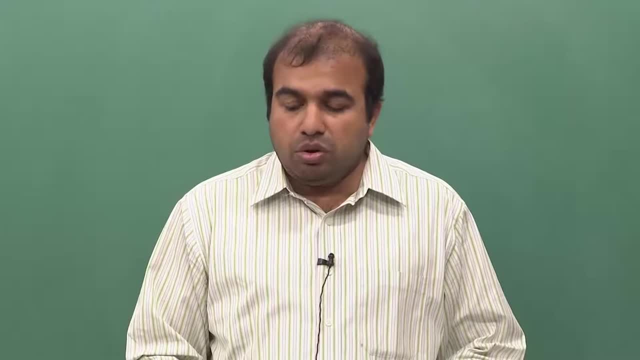 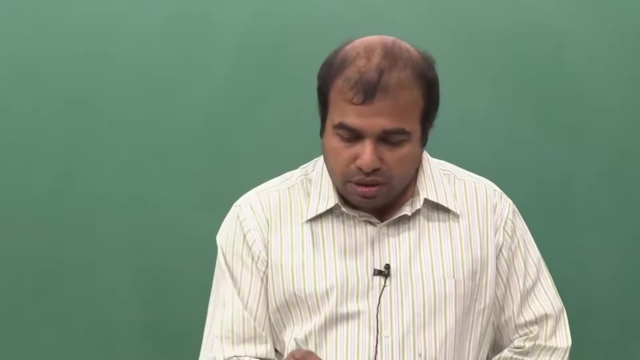 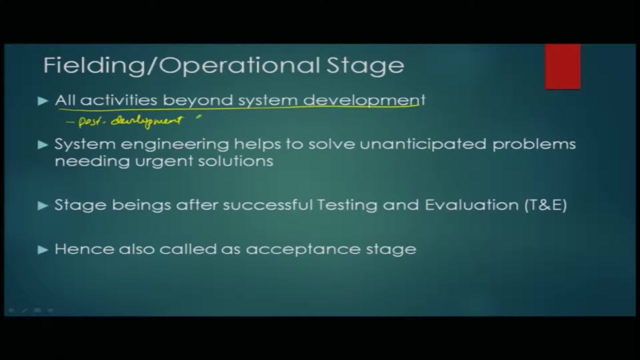 activities that are beyond the system development. So you are talking about everything that is after the system development. So what are the major things here? So the post development stage. some people call this as a post development stage, or some certain model calls this as post development stage. 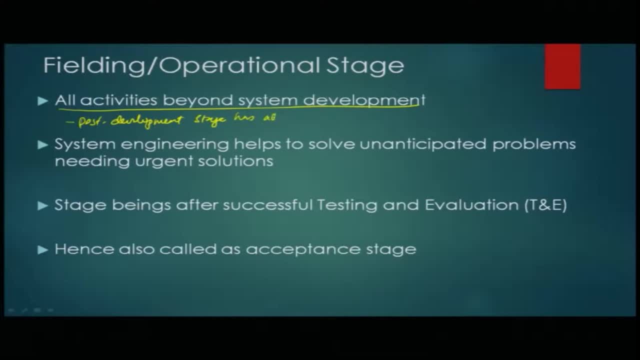 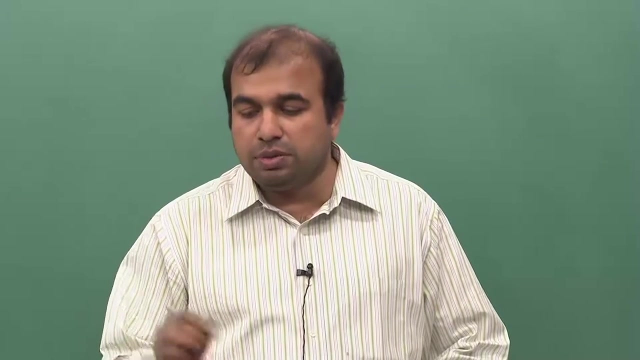 Post development stage has all activities beyond system development. but systems engineering is necessary. Why it is necessary? because it is necessary in supportive role. there are certain aspects after the development of the system, So systems engineering still needs to be involved in the post development stage of the system. 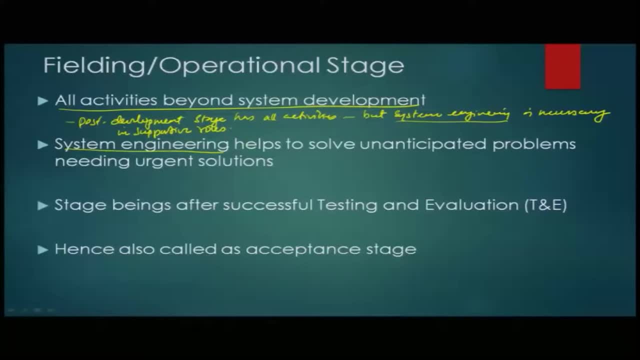 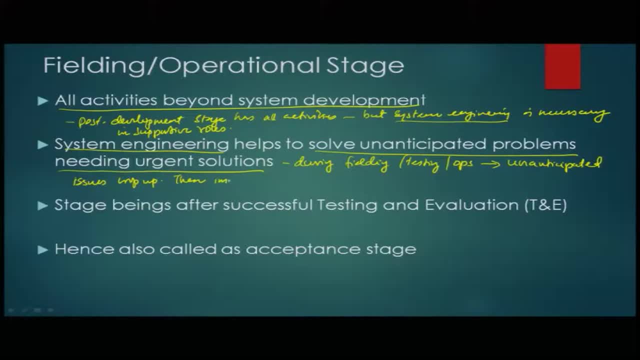 Okay, Okay, Okay, Okay, Okay, Then immediate resolution is necessary to continue or to ensure the continued usage of the system. We will discuss This Next. Next, discuss this point in little elaboration, using an example, real life example, later, during: 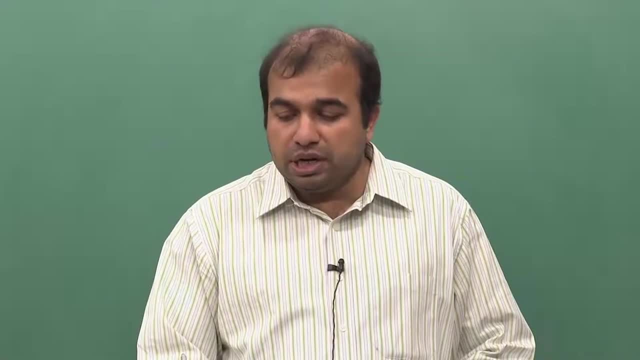 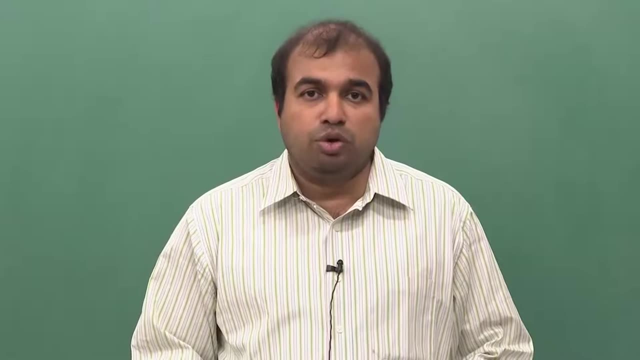 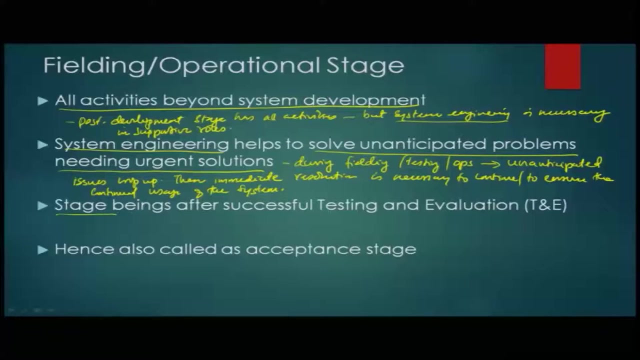 this presentation because it is important to stress this aspect, because many a times people do think that the fielding and operation stage, that all of the systems engineering, is not there. but systems engineering do play a significant or a major role in this process And also this is a stage at which successful testing and evaluation happens. 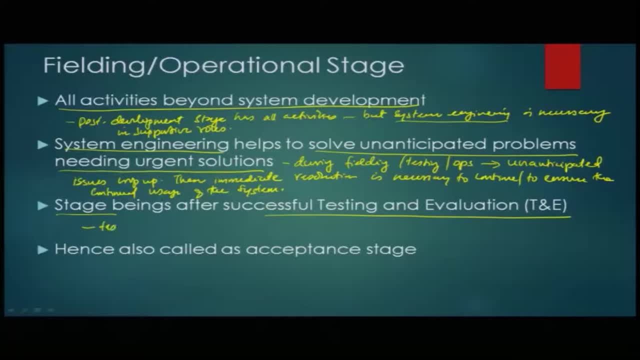 So the successful testing and evaluation means testing of the system in its operational environment, environment So that all desired functional capabilities Are demonstrated. So, as we mentioned in the previous slide, the test cases that are developed by the systems engineer comes in handy at this point, where the successful testing and evaluation, the 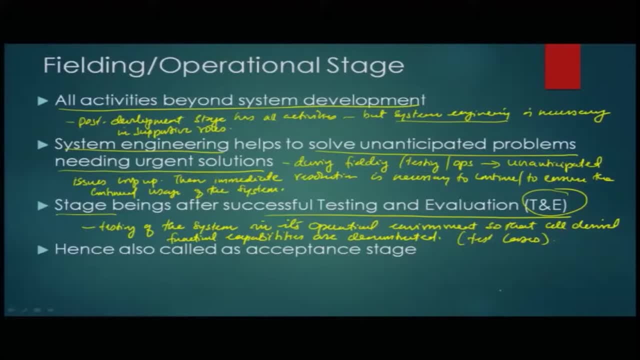 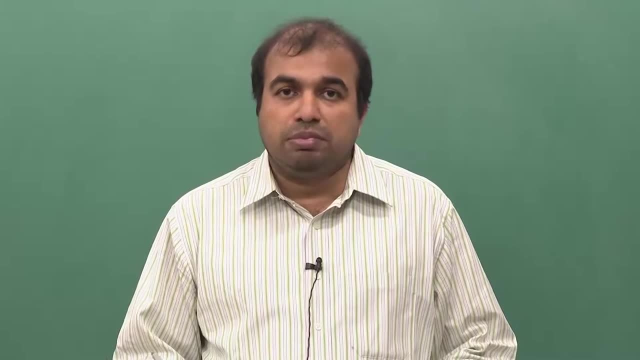 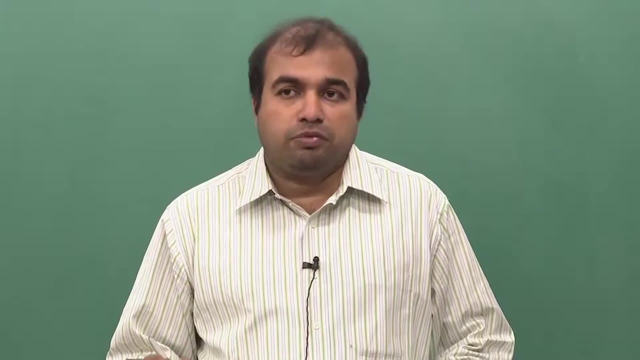 TNE of the system, where the user is taking the prototype, testing it, putting it into different test cases and seeing the performance of system and getting satisfied that all the functional requirements specified by the user Okay Is fulfilled by the design system or the physical design of the system, and that is why it is. 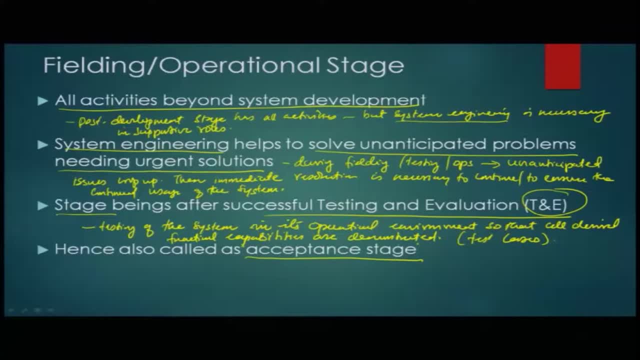 also called as the acceptance stage by certain people or certain model, certain systems engineering model developers, because this is where the customer accepts the physical design. physical design- that was The translation Of the concept, Of the system concept. Okay, So we also. another aspect of this is we should also think about it is the 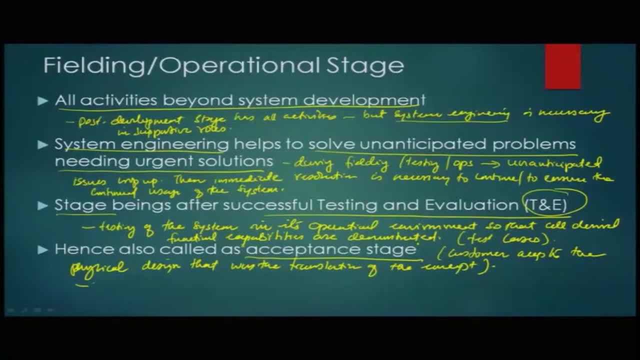 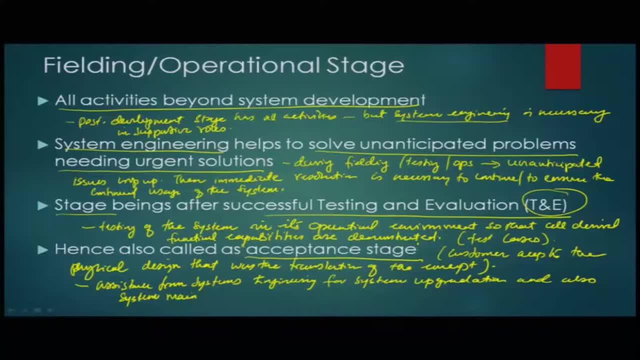 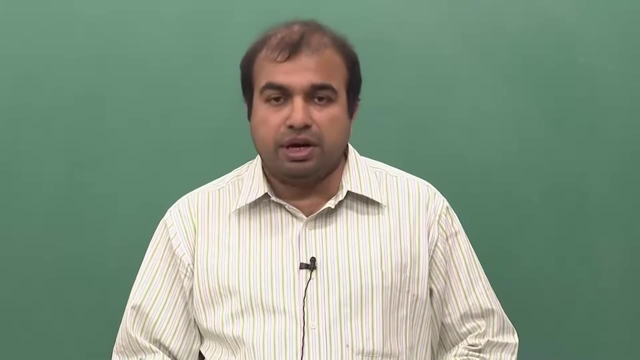 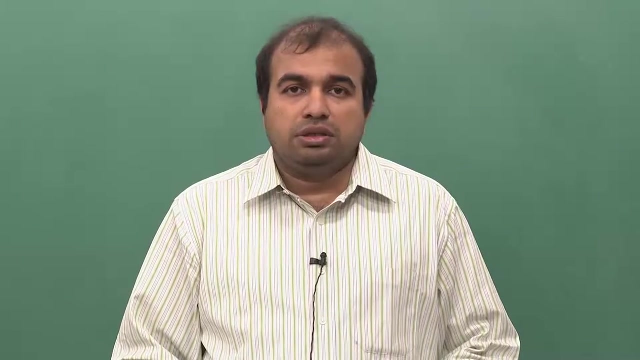 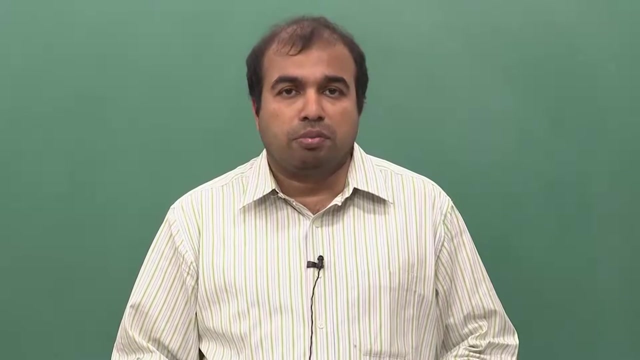 System Maintenance, Replacement. So, in addition to the testing, the acceptance testing of the system, the systems engineering help is also needed for upgradation of the system because some of the things that might when the user uses this- oh well, this is really good- but it has taken some time to develop the system because, remember we already told that all systems engineering projects are usually long projects because of the complexity of the systems involved. 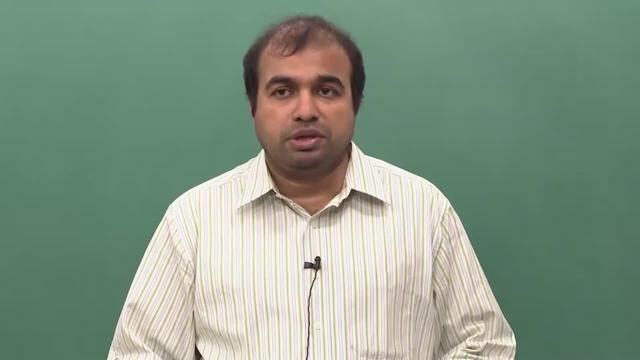 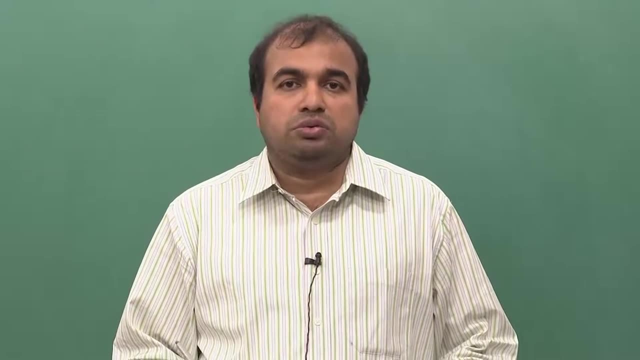 We are talking about development of systems, of systems or complex systems. So it is not a one or two year project. it probably be as long as five, eight year long project. So during that project the technology would have advanced And when the system actually come up, 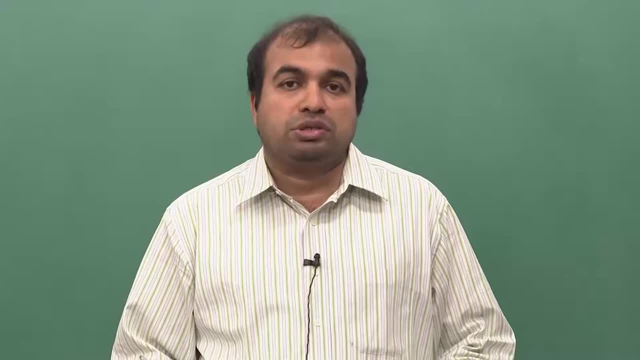 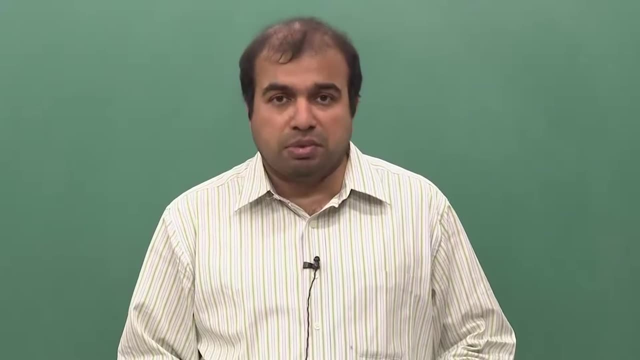 The user feels that, okay, this is a new thing that need to be happened. so the system, also the current system that need to be developed, Need to be Upgraded to suit that. So that will be one aspect of The systems engineering where the systems engineering will also help. The last and final aspect will also be the Supply chain management, The systems engineering or systems engineer. help is required in also maintaining the supply chain to ensure that the product fulfills its operational life cycle. So that is also needed because during the life cycle, parts need to be changed, things has to be maintained. all that requires a dedicated supply chain or a smooth functioning supply chain. that is required. 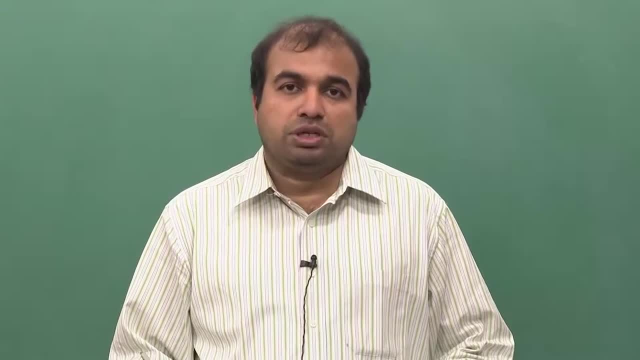 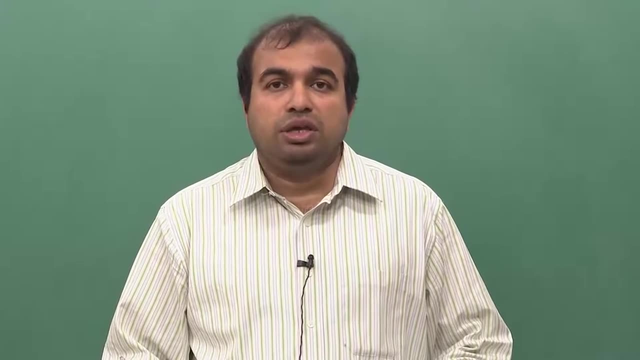 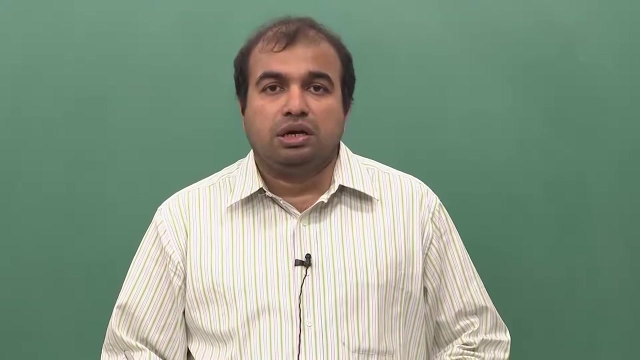 Which should also be, Which is also the responsibility of the systems engineer, to design the supply chain and make the user aware of such a supply chain so that the user, when he use, when the user utilizes the system, It can utilize the supply chain to ensure that the system continues to operate successfully throughout its entire designed life cycle. 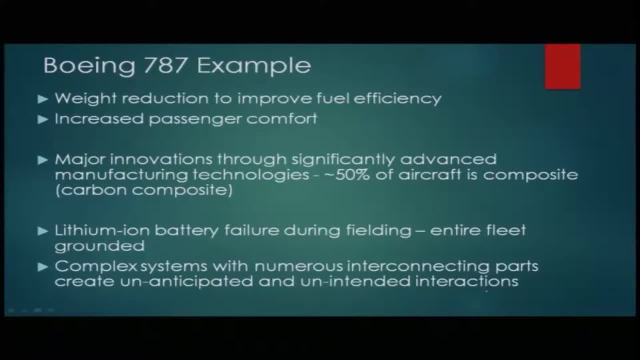 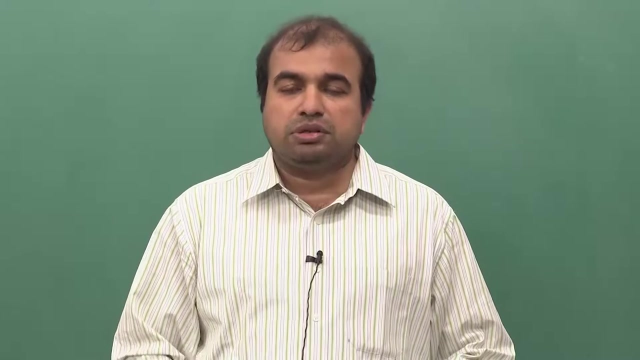 So let us talk about an example to discuss about these aspects: The Boeing 787, or what is commonly known as the Boeing 787.. Or what is commonly known as the Boeing 787.. Or what is commonly known as the Wolverine, what is commonly known as the 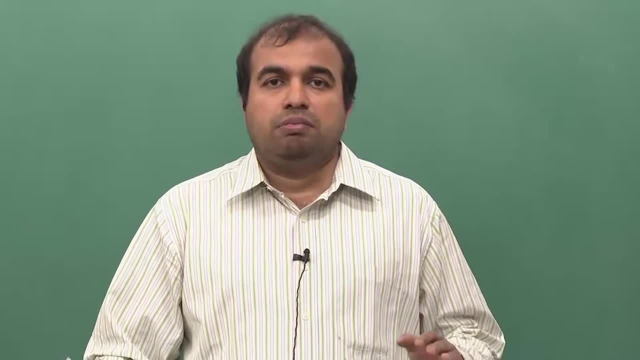 Dreamliner, For example. There is quite it's a quote along big example, but what we will try to do is we will try to take some simple salient points and try to establish The importance of systems engineering and how the systems engineering did actually help after the productivity was filtered. 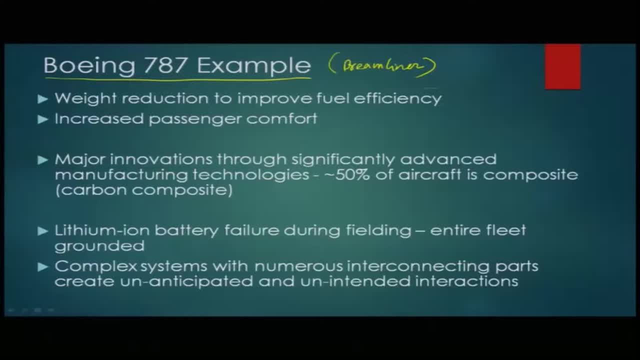 So the main, there are many aims, so. So this just Just to knows, If you want a поговор in it a bit. Yes, just two representative requirements of 787. I just took this just to demonstrate things. there are so many multiple, many, many, many requirements that were part of the 787 design. 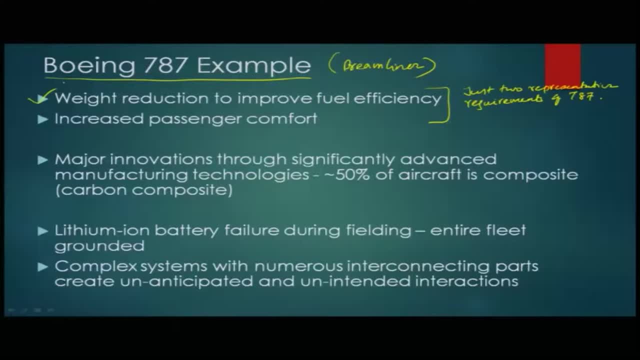 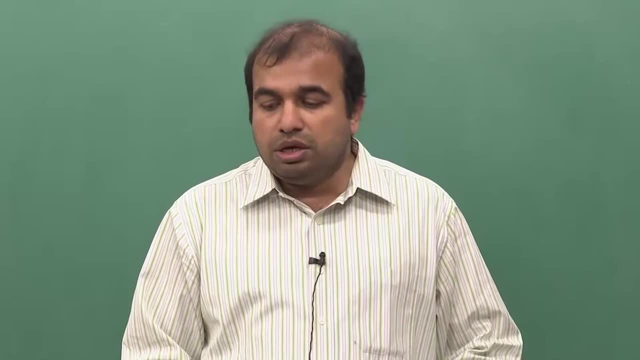 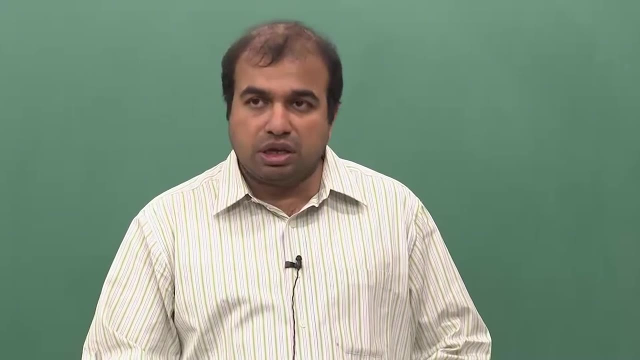 but two important things that we talked about here was the weight reduction to improve the fuel efficiency. So the Boeing really wanted to reduce the weight of the aircraft because if you know, for anybody who is in the aerospace engineering would know that any aircraft that need to fly or that that flies over any body that flies, you know that the thrust should. be equal to drag and lift should be equal to weight. So if the weight reduces, then the requirement of the lift also reduces. when the requirement of the lift reduces, then the amount of thrust reduces. So the aim was to actually create an aircraft that has less thrust requirement but can carry. 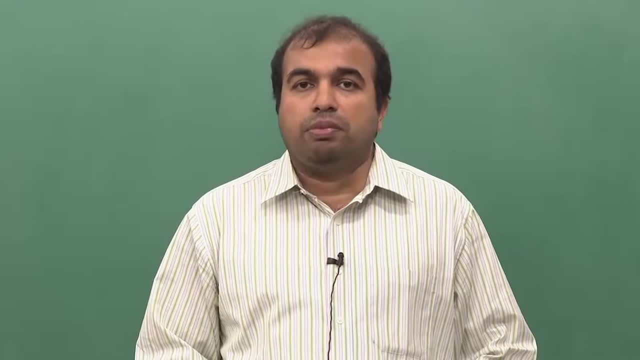 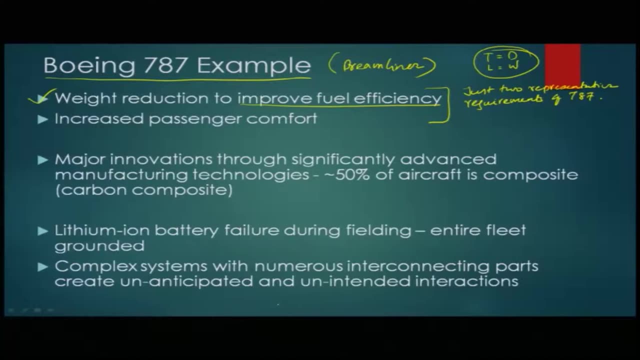 thrust requirement due to its less in less structural weight, So that you can get a better fuel efficiency out of it or improved fuel efficiency out of it. and second goal was to increase the passenger comfort or comfort in a such sense that reduce vibrations, reduce. 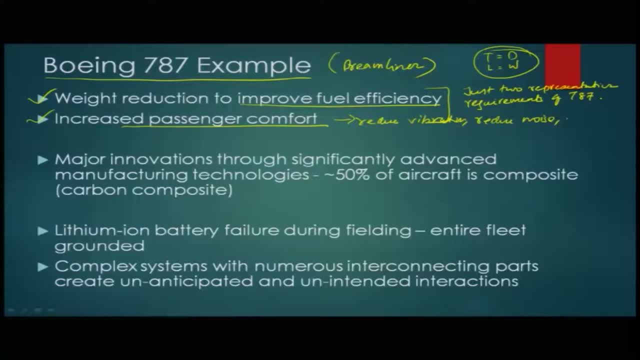 noise, etcetera. These were the some of the aspects of the two aspects of the Boeing Dreamliner 787.. There were so many more other more aspects, but we are not talking about that. we just taking two as an example. So one thing: when they started designing this and developing this, they found out that the 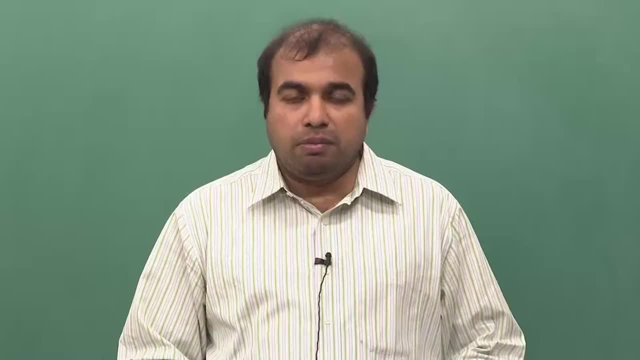 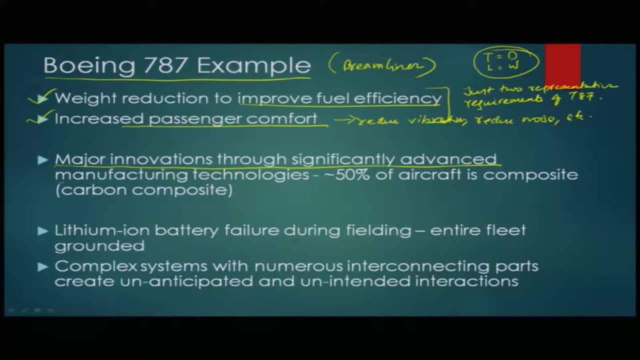 technology is not there to actually develop the airframe using composite materials. So major innovations through 787.. So this is where we talk about the identify new tech. that is part of the concept phase- was figured out that if the aircraft has to be built, about 50 percent of the aircraft 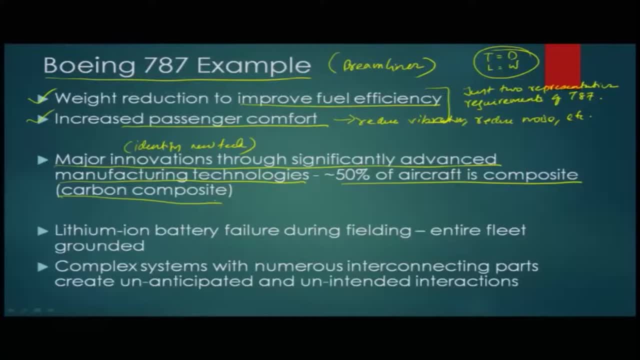 is to be composite or carbon composite based aircraft. for why? for what? reducing the weight, the reduction of weight. this was the option that Boeing took, because if you want to reduce the weight, So a significant portion of the aircraft need to be built using composites. and if you 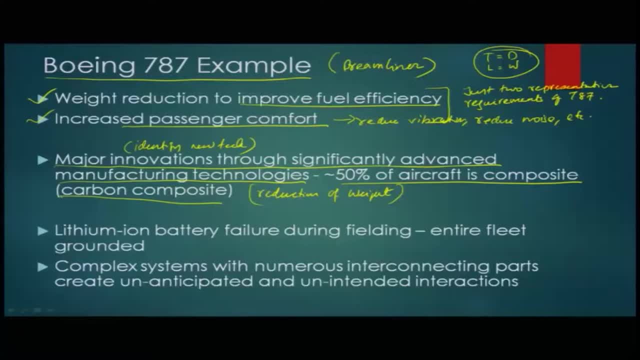 have to build the aircraft using composite. you have to build advanced manufacturing technologies that were not available at that point of time. So Boeing invested in developing the new advanced manufacturing technology to realize an aircraft where approximately 50 percent of the aircraft is composite based. 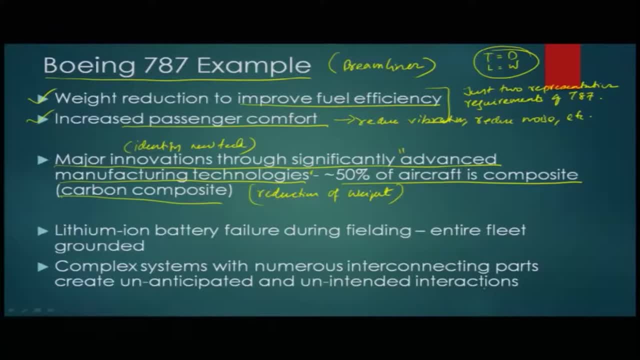 So this is where, then, they just did not develop the manufacturing stuff. they developed it, tested it. So this is where, then, they just did not develop the manufacturing stuff. they developed it, tested it and validated it. The new manufacturing process has been developed, tested and validated. 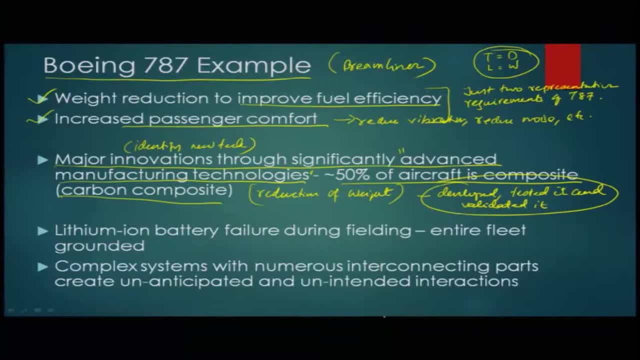 So that was one aspect of how the new technology gets developed as part of the concept phase. But then the dreamliner came out. it became a big hit. lot of companies ordered. significant amount of large ordering happens because the improved fuel efficiency- lounge area efficiency- translates to significantly lower operational costs. 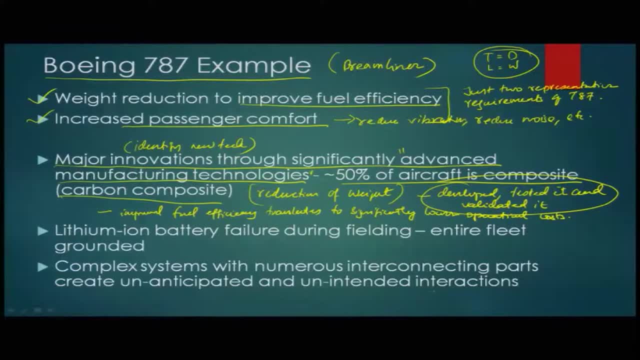 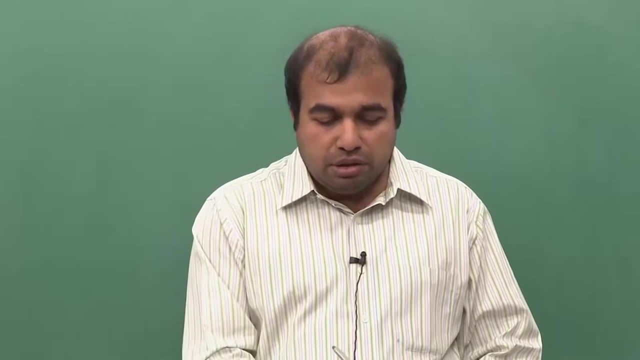 So everybody felt that Boeing 787 Dreamliner is going to be a big hit. it is going to revolutionize the entire the way in which aviation sector is going to perform. So it was. it set up a new benchmark. Everything was going great until one point of time. the problem that almost everybody 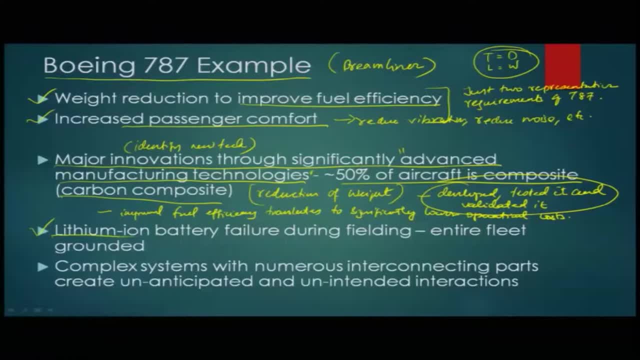 anybody who is to deal with engineering might have heard about this: the lithium ion battery failure during fielding of the 787 Dreamliner. you might have heard about the case of ANA or the Nippon Airlines, all Nippon Airlines, the Japanese Airlines. Here, the batteries bursted during flight, creating significant, significantly dangerous situation for the passengers. it So the lithium ion batteries that were used in the Dreamliner 787 started behaving badly and when multiple aircrafts had the issues, batteries started bursting. then the FAA 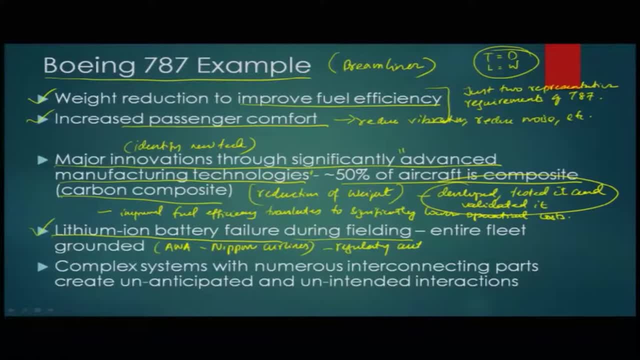 the regulatory authority authority Flight Like FAA and all issued warning that the fleet needs to be grounded. So anybody who was operating the Dreamliner 787 had to ground the fleet up to how far until Boeing solves the problem. So then the Boeing system called upon a systems engineers. 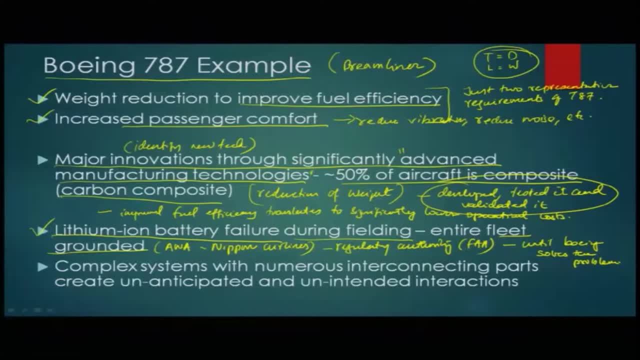 To figure out what happened. and obviously we know that if you are engineering a complex system like an aircraft, like a Dreamliner, there will be so many numerous interconnecting parts, myriads of interconnecting parts, And when all these parts are interconnected, there are many parts are interconnecting. 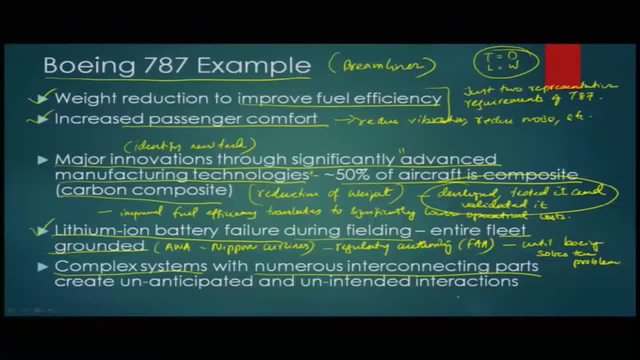 then you would try to you think that you taken care of all the cases. But many times there will be unanticipated and unintended interactions between the systems. So the systems engineer might have developed test cases for validating things, but at a one particular point where a specific combination of temperature, pressure and other aspects 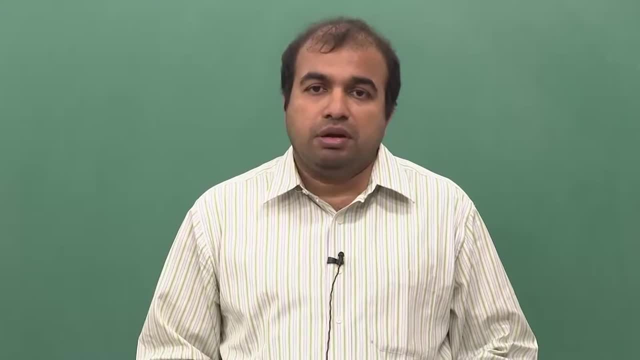 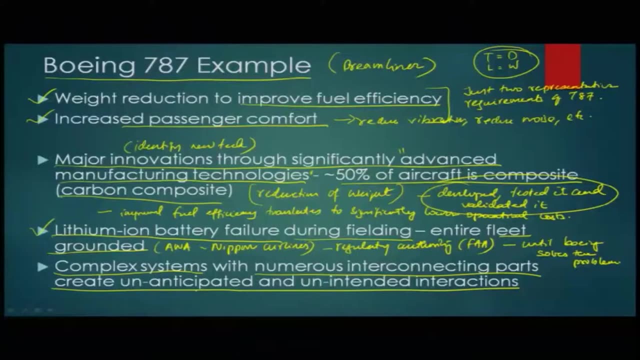 came in, or a condensation came in or moisture level came in, the batteries behaved weirdly. So one of the major reason at this point, or the reason for this failure, was that the interactions or the interconnecting, Interconnecting, Interconnecting, Interconnecting. 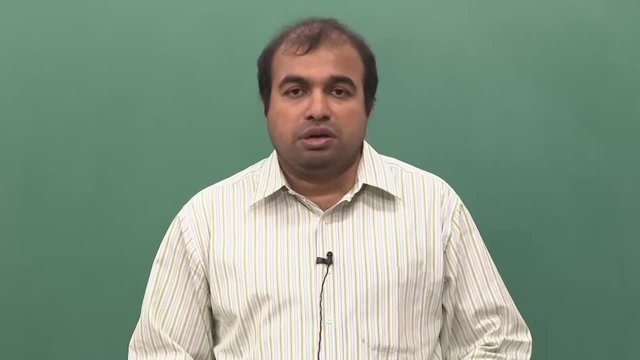 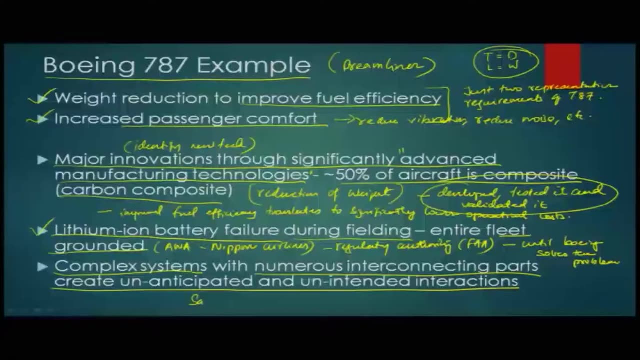 In the complex system. the power management system of Dreamliner was causing the problem, And same system, same behavior was also found in another example would be Samsung Galaxy Note 7.. So, anyway, Boeing got into the act together and got the- you know systems engineers to 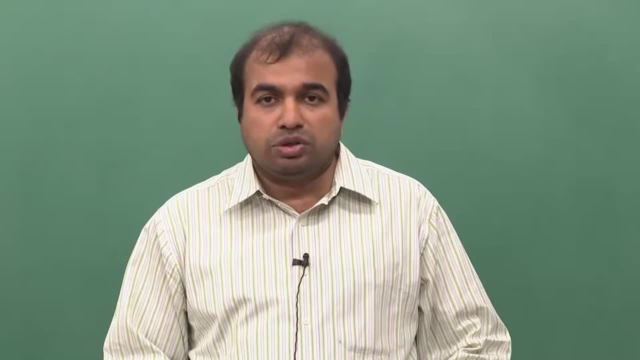 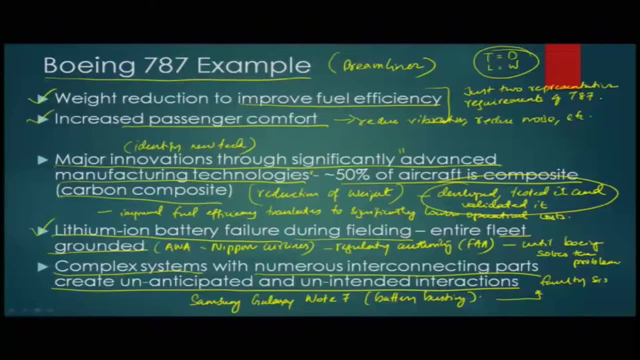 come up with an alternative approach, design of interface, come up with better choices of batteries, and then the faulty situation was rectified. Once the rectification happened, testing continued, then certification again was done and then the fleets were back into normal. So this is a particular situation where the systems engineering was called in again to 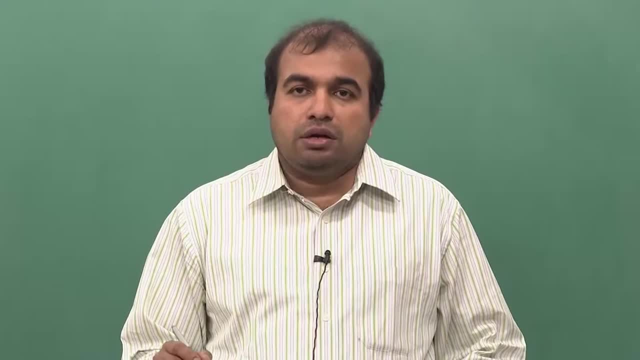 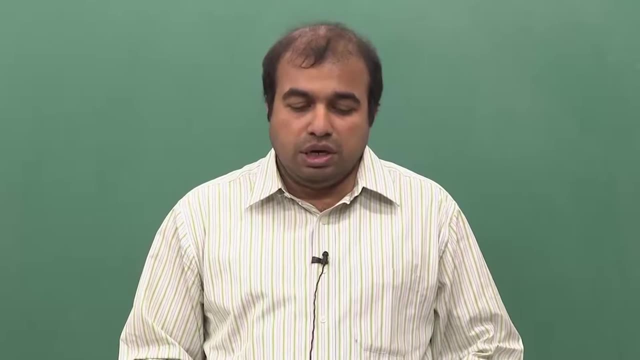 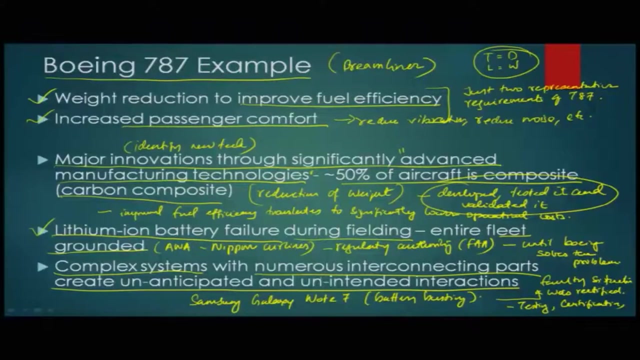 assess the fielding of the fleet or the operation of the Dreamliner 787 during its what we call as the deployment phase, or when it is actually fielded. So if the take away from this example is that it is not just the, so you can think about. 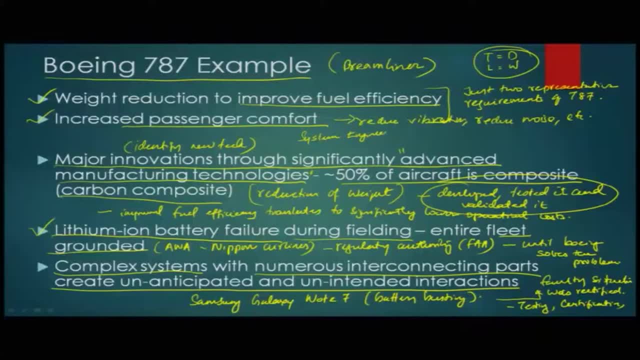 this way, Systems engineering. Systems engineering is obviously needed during development phases, the two development phases, the concept phase and the engineering concept and engineering phases, but it is also necessary during the development phase, The post development phase or the deployment phase of the system. 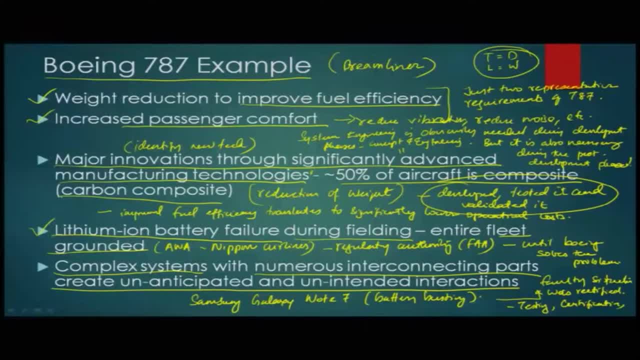 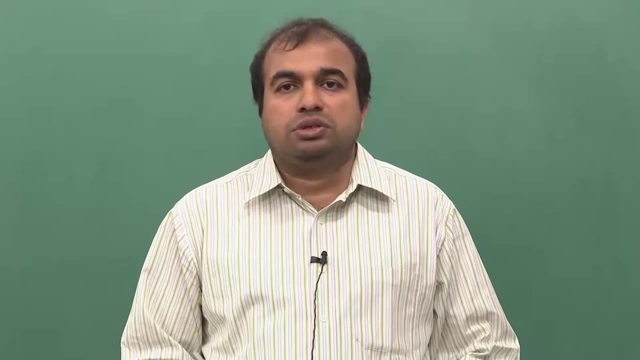 So that is also an important take away of the exam of this lecture or of this example, is that any system, any complex system, when you engineer you will, it will be almost impossible to develop test cases, to test and validate every aspects of the system. And given the fact that Boeing designed Dreamliner 787 and there was only one major issue with the battery and one minor issue about the door or the issues with the hinges of the door, Other than that, having just two issues that need to be sorted out in the design and development, 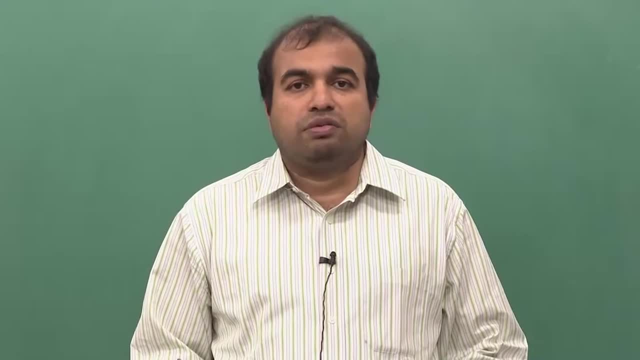 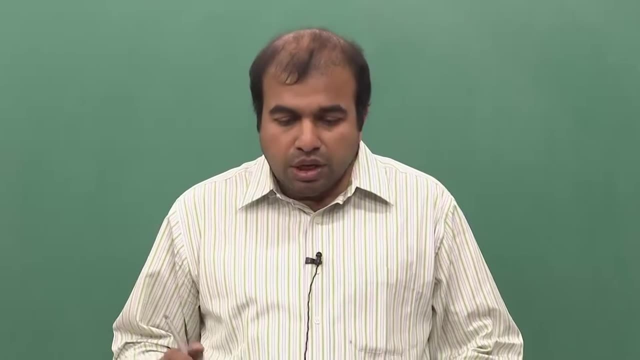 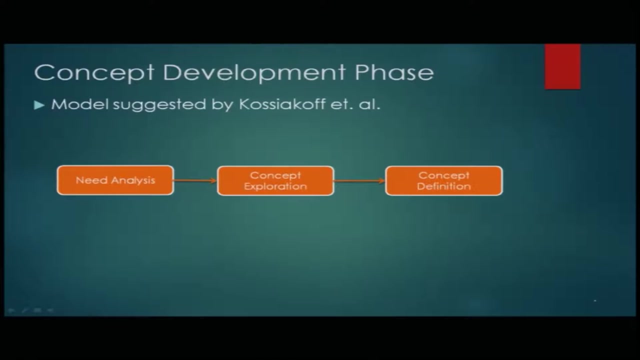 of such a complex system shows the importance or the significance of going through a good sound systems engineering approach. Thank you, So we will look into the further details of the systems. the concept development phase, which is model, is proposed by Kosayakoff et al. 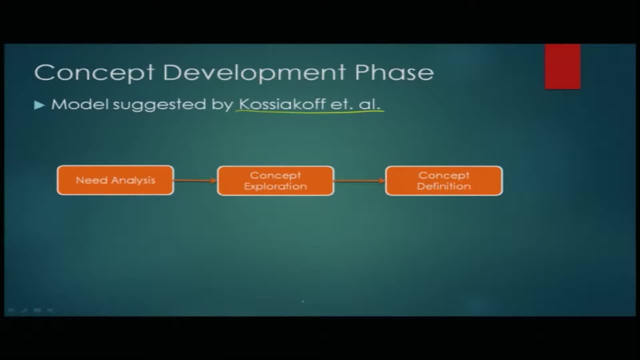 And their specified different aspects of it, which also gives you a very good overview of what are the inputs and outputs of each of the processes of the system. So the first phase, which is a concept development phase, as we said earlier, has three important 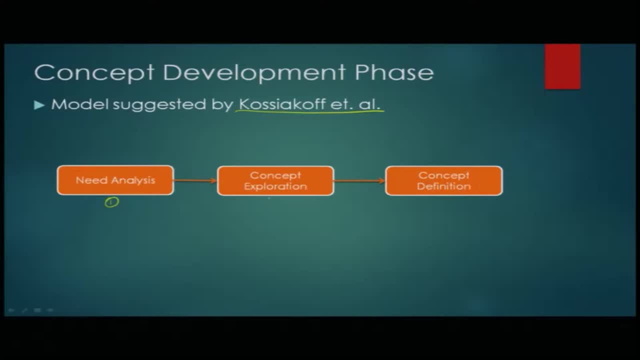 steps in it need analysis, which is the first step. second step is the concept exploration and third one is the definition. So the need analysis has typically two inputs. The first input comes from the operational deficiencies. that is the first aspect. The second aspect comes from the technological opportunities. 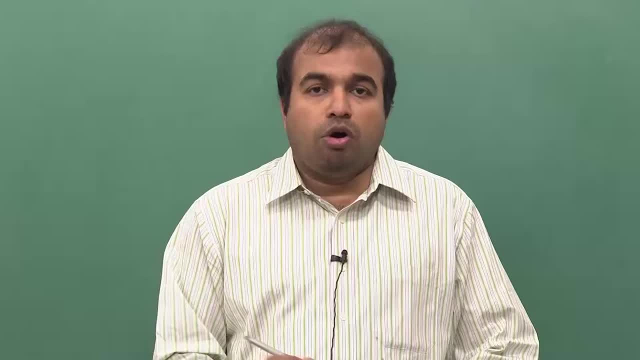 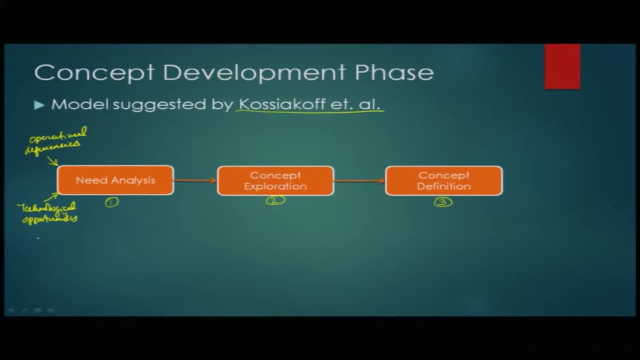 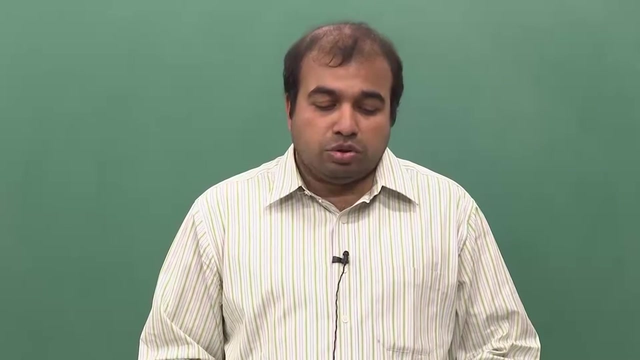 So the two inputs, the technological advancements, give you a new option. So, as I said earlier, how nuclear submarines arrived, because it is a technological advancements in miniaturizing the nuclear reactors suggested the feasibility of developing a nuclear submarine. Similarly also the operational deficiencies. 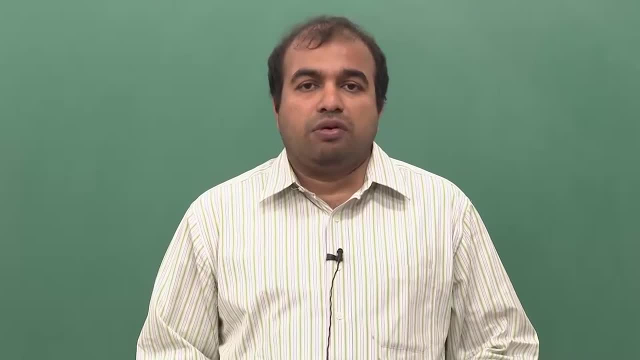 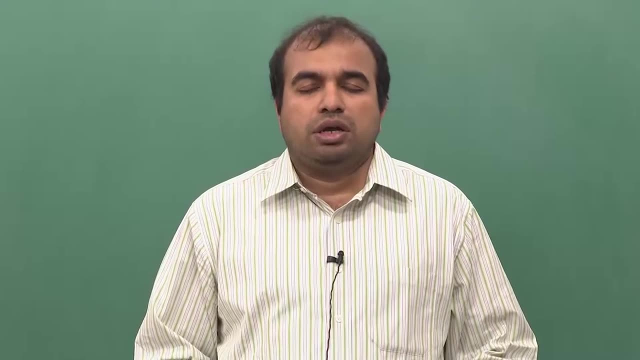 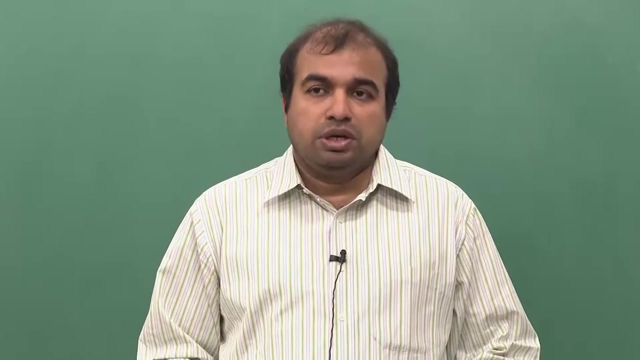 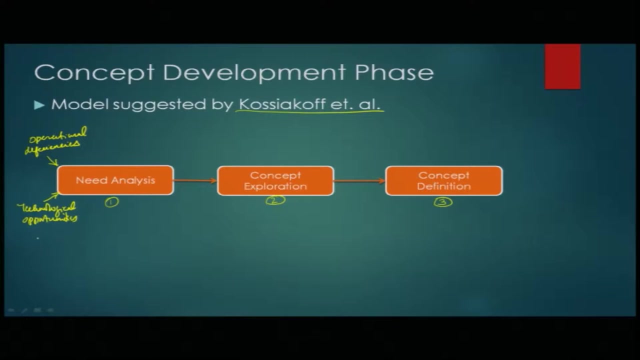 Like. an example of that would be India looking for medium range fighters because of the depleting field- sorry, depleting fleet conditions of the air force has forced India to actually look for stop by arrangements. So that is an operational deficiency. So sometimes operational deficiency, sometimes a technological advancements, sometimes both. 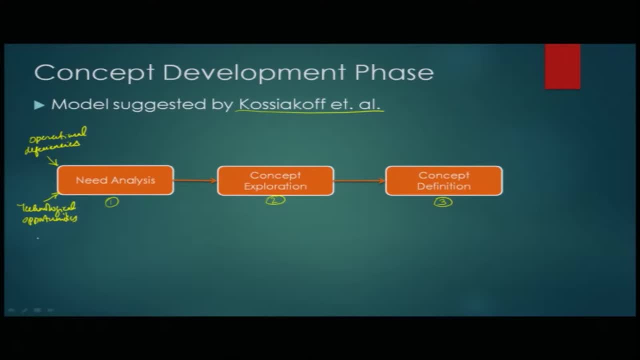 of them put together creates a need or establish a. So both of them put together creates a need or establish a. So both of them put together creates a need or establish a. So both of these- here you are talking about the need- is a valid need for the customer. 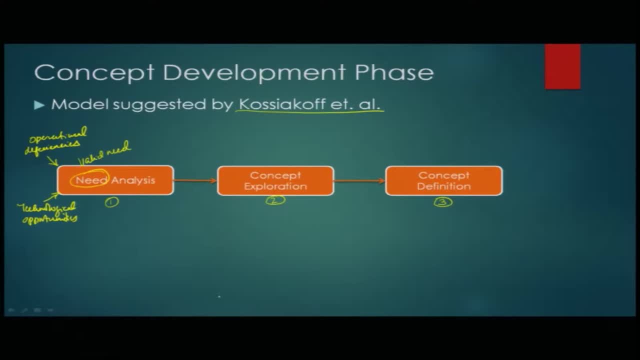 So once that comes in, then from there, multiple things happens within this. So what are the major multiple things happen within this? The first one will be the system studies. So multiple studies will be undertaken to study what are the possible system. Then the second one will be the 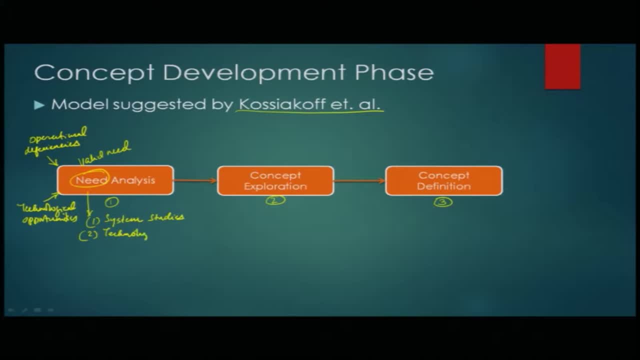 Then the third one will be the technology: assignment assessments, not assignment assessments. So here the readiness, technological readiness, is being assessed, whether the technology is available or is the new technology need to be developed. All those aspects comes out here, and then the third aspect will be operational analysis. 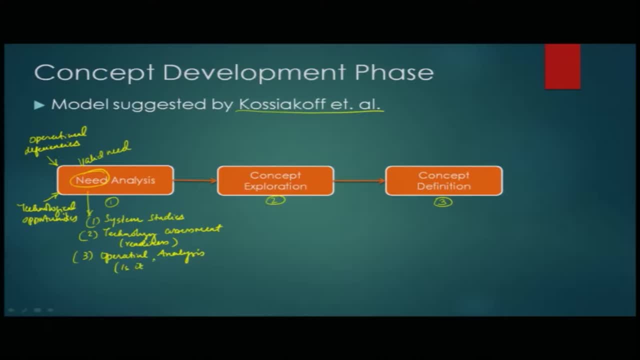 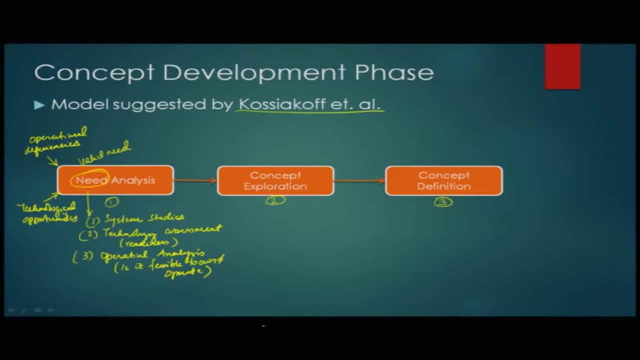 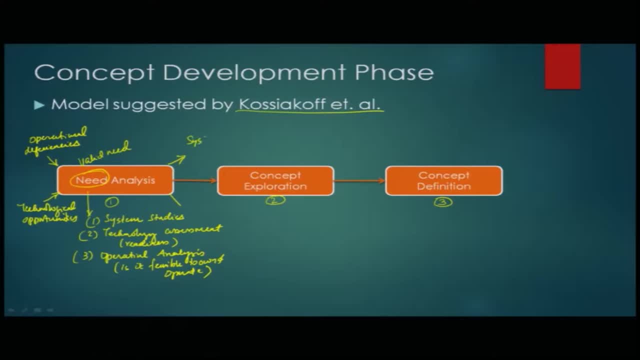 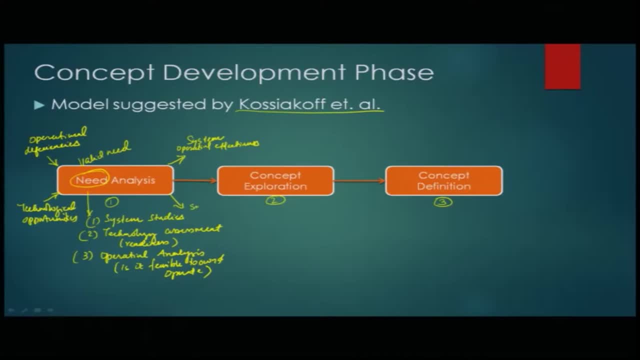 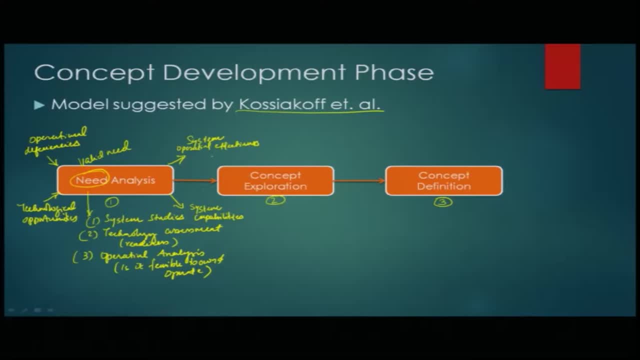 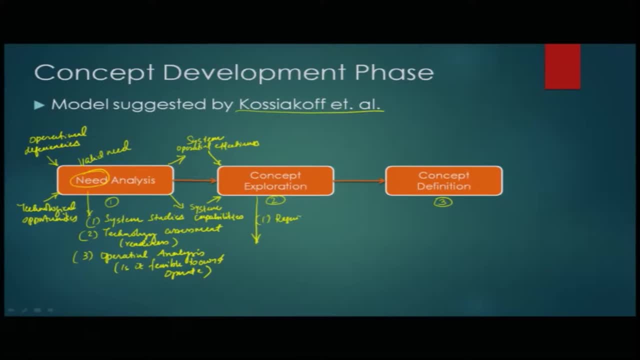 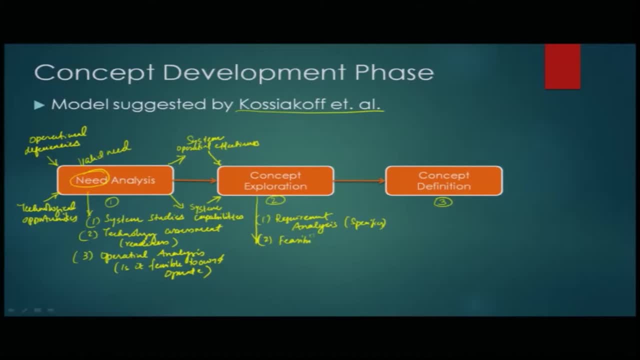 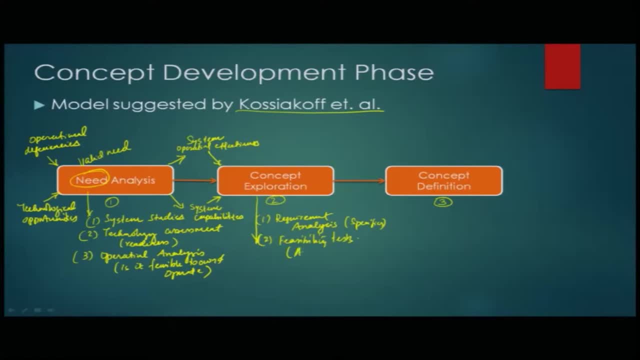 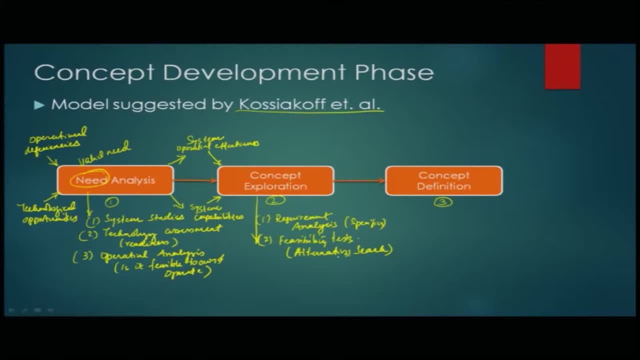 Is it possible to get? Is it possible? Is it feasible? Is it possible? Is it feasible? What we want, bro, Think about something. wasn't it a possible weights weight, What you came out to be? You brought in the. I wanted the weight. less than that. 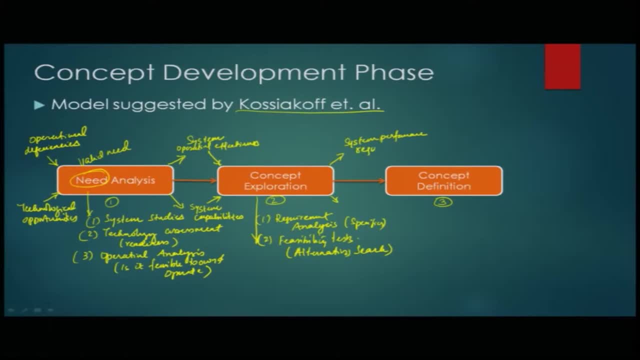 Increased the weight from the load Ease, so that what else you want to do in terms Okay, so thank you, bye. You don't want to go on in terms of B noget, So let's go with that. B gibt To performance requirements, so not just the so specific performance requirements. 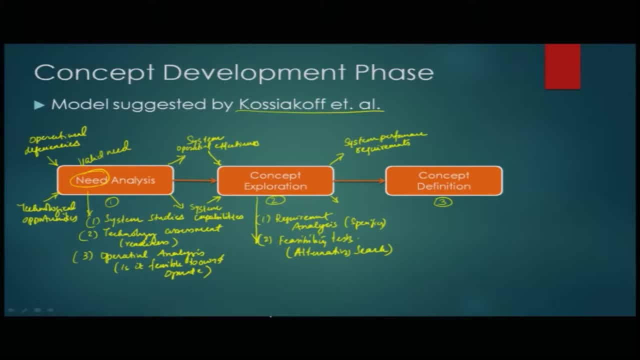 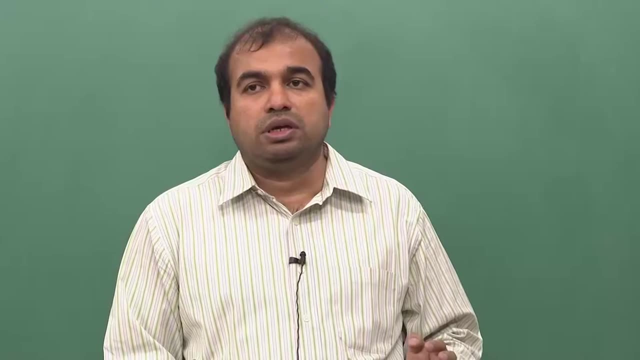 So, like, for example, in the case of dreamliner, what we talked about one of the performance requirement will be: 50 percent of the aircraft will be built using composite, resulting in a weight resulting in a 20 percent less structural weight, or it could be like because of the 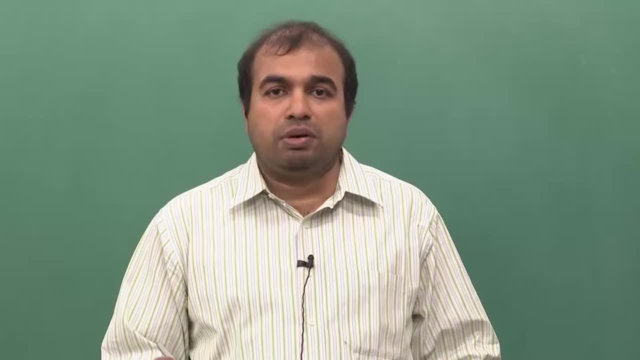 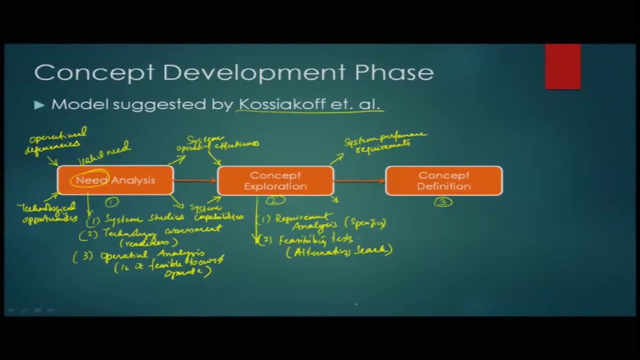 less structural weight. the thrust requirement is reduced by 10 percent, resulting in a fuel efficiency increase of 3 percent. So something like that. the specific performance requirements will get actually crystallized as part of this, and then the second aspect will be system concepts, multiple system concepts. 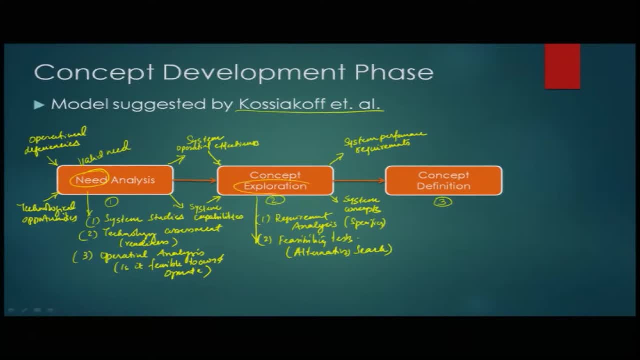 gets derived as part of this. So here you are, exploring. the exploration is the big word here. Once the exploration happens and the performance requirements comes out, which becomes the input to the third phase, which is the concept definition. and the concept definition is where basically two aspects happen. 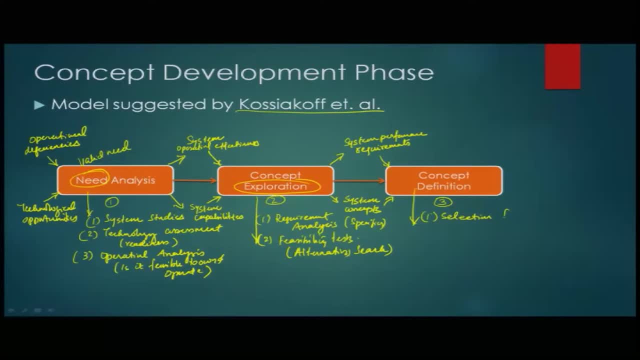 First is the selection from alternatives, or you can think about it as trade-off studies. how are you doing different trade-offs among different alternatives? the positives and negatives of all or possible alternative system configurations are evaluated So that an appropriate system can be chosen out of that. then the second aspect of this. 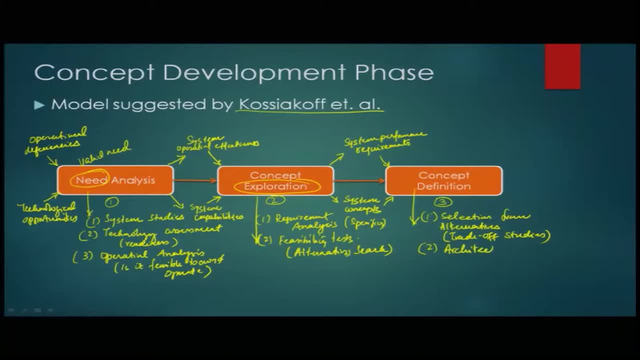 will be the architecture, Not talking about the. it is called as a system architecture. Please remember that this is not engineering architecture. not is the keyword, not engineering architecture, But here, in one of the earliest presentations, I have mentioned that it is mostly related to the engineering architecture. 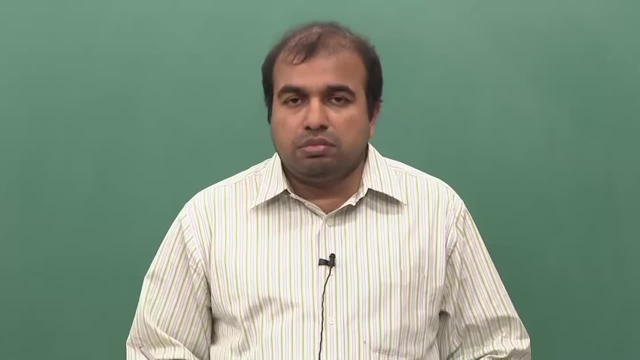 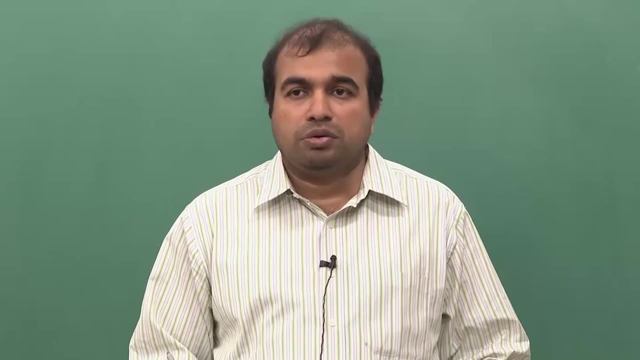 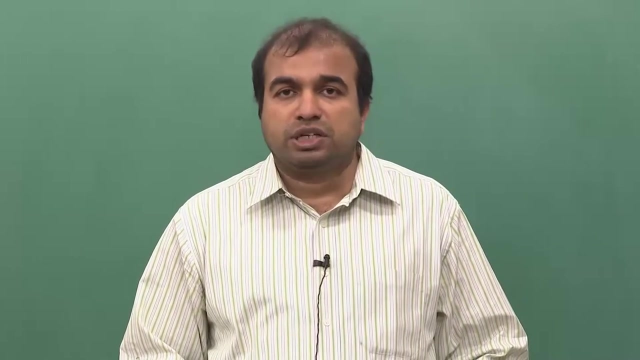 Okay, So it is not the block diagrams and interconnectivity and those kind of aspects, not just specifically choosing what will be the specific component, that will go into it. Sometimes some competent information is available, but not necessarily because lot of that- competent choices and other things- will be the job of the experts, not the job of the systems engineer. 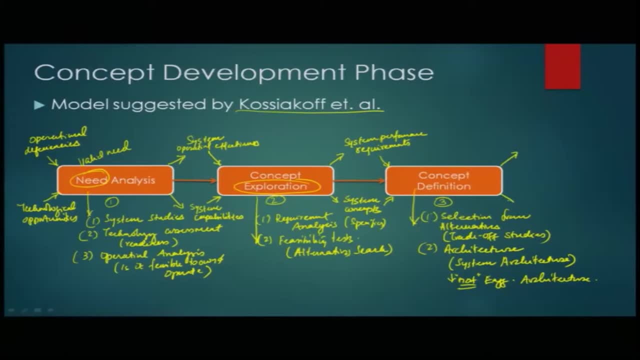 at this phase. So out from here we get two outputs. two major outputs comes out of this, and the two major outputs of the system are Okay. These are system functional specs specifications and system concept definition. So here you can think about it as a chosen system. 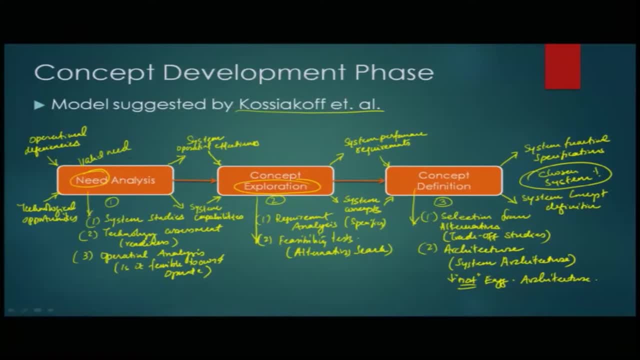 So one single system is chosen here, and then the functional specifications of the chosen system, Okay, And as well as the concept of the chosen system gets specified as part of the output of the stage. So, summing up again, the three phases has the analysis of the needs, where the valid 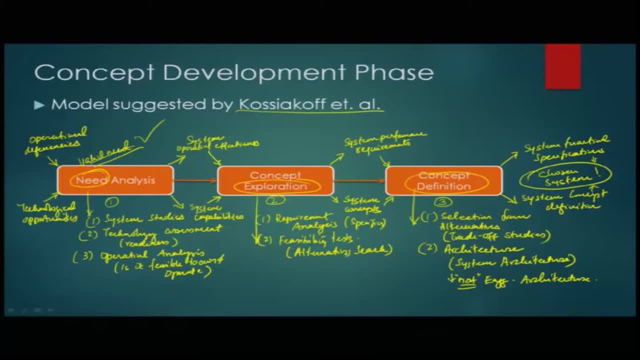 need, validity of the need of the customer is established here and from there the capabilities, the required capabilities of the system and the operational effectiveness are established, which goes into exploration. Okay, So multiple systems are multiple, alternatives are explored, their aspects are listed out, from where the system performance requirements and the concepts- both of them come out as: 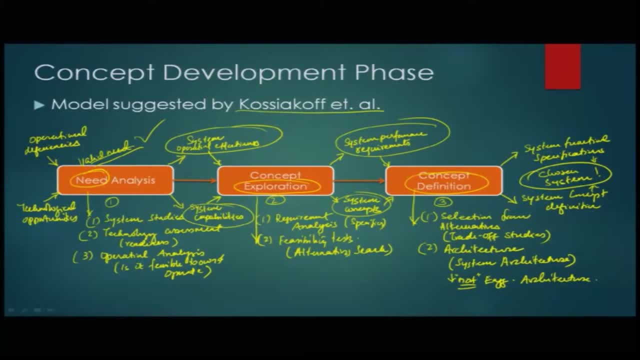 output of it, which gets us the input into the third stage, where the appropriate choice of the system is done or a specific system is chosen from there, and then the functional specifications of the chosen design and the concept definition are both as part of comes out as the output of this concept development. 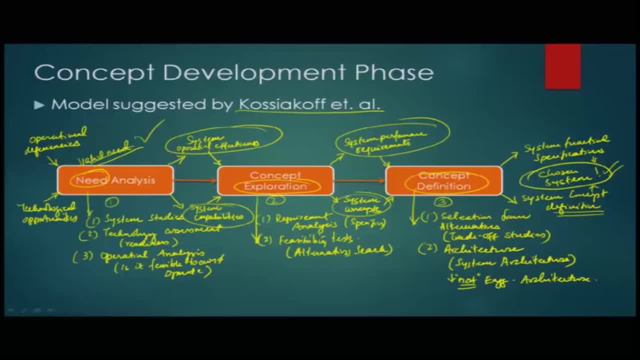 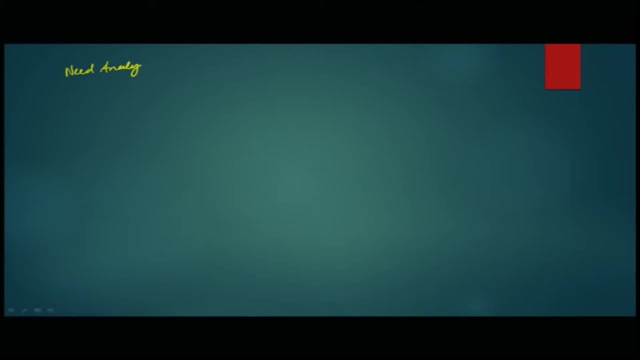 The concept development phase. Also, we should understand the fact that when we talk about need analysis initially, what do we do there? So need to remember these two important questions: Is there a valid need for a new system? This question is the first and foremost most important aspect that becomes a part of the 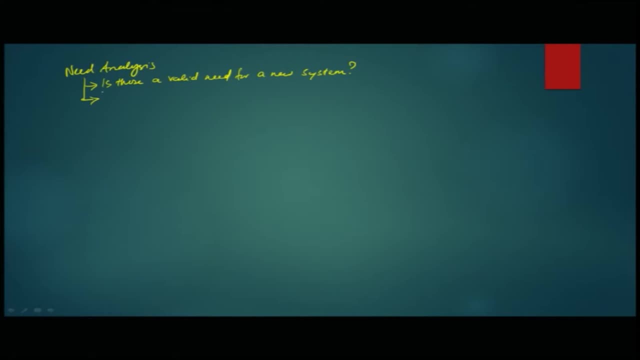 need analysis. The second important question is the: is there exist a practical approach to satisfy the user need, user need for a new system? Okay, Okay. So the two important aspects that gets covered in the need analysis is: is there a validity of the need for a new system? does the customer require a new system and is there a practical 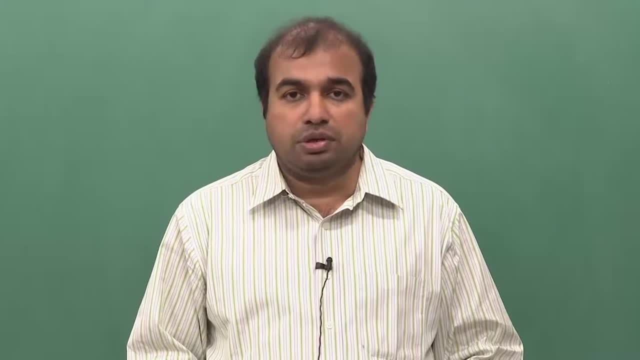 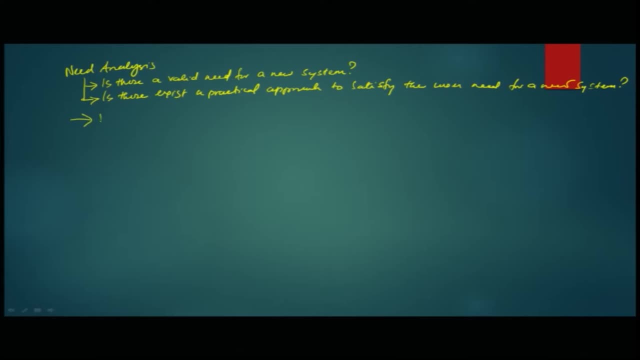 approach available to satisfy the user need for a new system. is it feasible, can be made, can be built? So, in a way, the output of this is the first iteration of the system itself. Okay, Okay. So in a way, the output of this is the first iteration of the system itself, which obviously 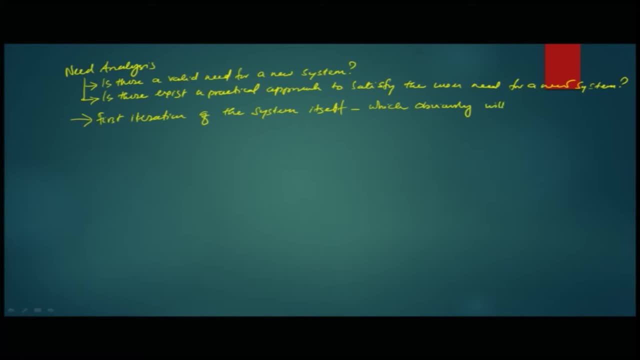 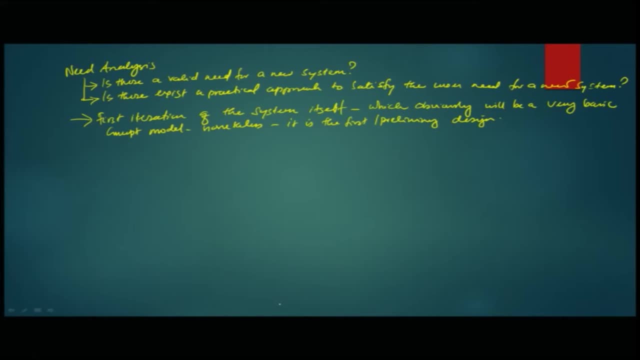 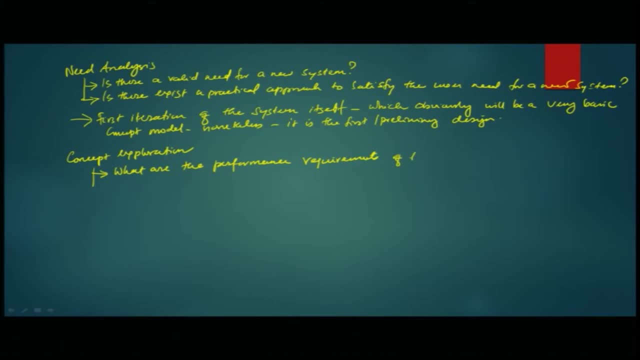 of the new system, of the new system, so that user needs can be satisfied. That is the first question. The second question is: is there at least one feasible approach, approach to achieve the desired performance, desired performance, performance at affordability? 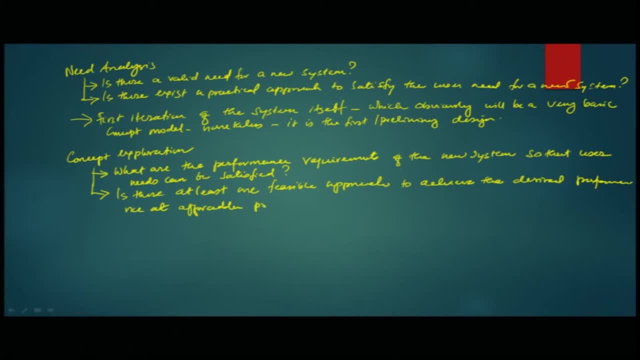 Affordable cost or at affordable price. So the two aspects you are looking at: what are the possible options, what are the performance requirements of the new system so that the user needs can be fulfilled, and what are the feasible approaches to achieve that desired performance at an affordable price? 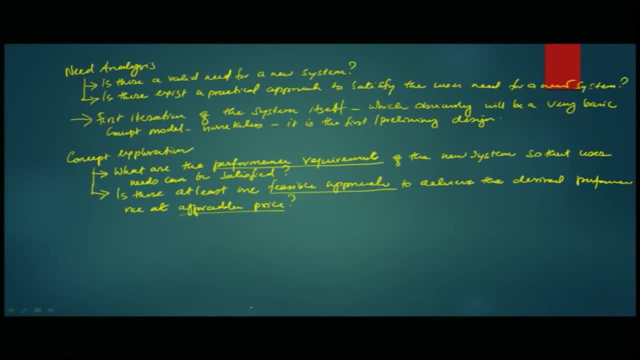 So that will be the aspect of the concept exploration and the some of the tools that are used in concept exploration. So the concept explore tools involve various process methods, decision support systems, expert analysis. also Delphi method, etcetera are all part of this. 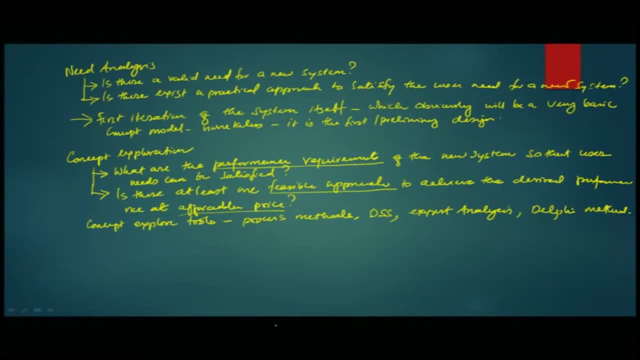 So multiple tools are used so that different feasible approaches can be thought through. so your expectations: Exploring the concepts. Then comes the definition. the concept definition, the third aspect, And here the major question, the single question that gets answered here is: what are the key? 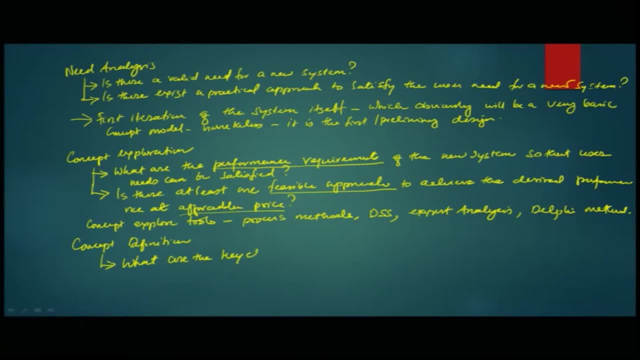 characteristics, characteristics of a system or of the system concept- That can provide the best balance. we earlier talked about the systems. engineering is a balancing act, the best balance between capability, capability of the system, capability, life of the system and cost of the system. 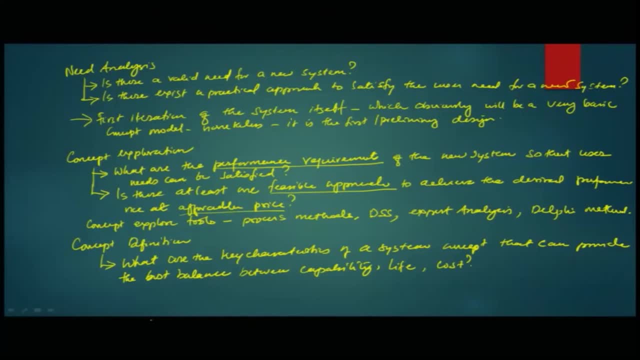 So this is the major question, So the functional specs. so here in this regard is the. as we said earlier, the output of this whole process will be the functional specs For specifications, which means it is a description of what the system must do and how it will be. 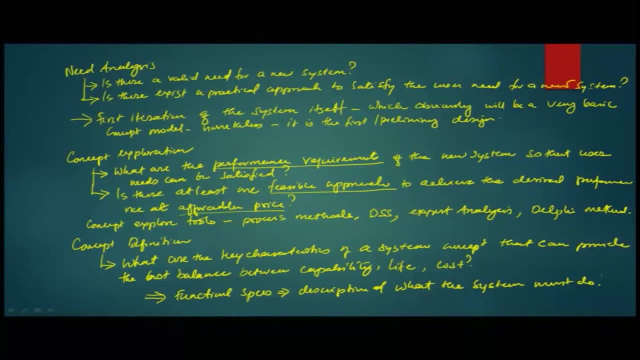 able to differentiate between different, different systems. right, These are the 3. You have use ored ca speaks. how well is the aspect? So the functional specs basically provide, at the end of this whole exercise, what the system must do and how well is specified as part of this, and